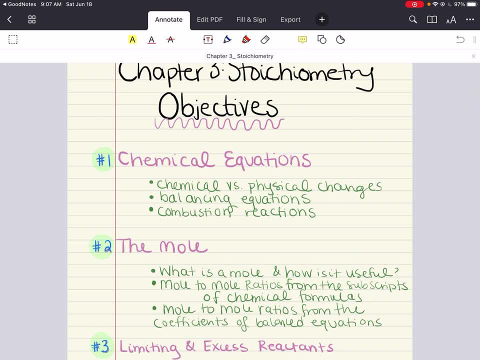 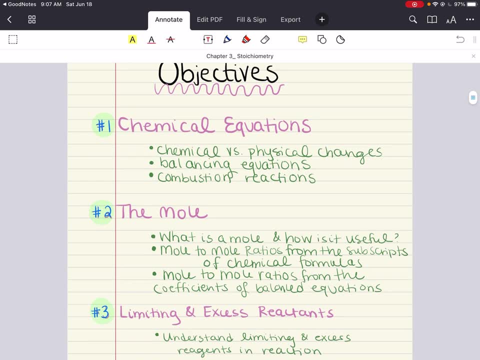 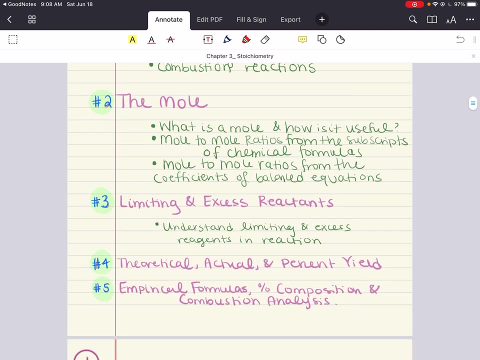 equations, specifically learning how to balance chemical equations. Second, we will talk about a unit of measurement called the mole, and we're going to discuss how we can use this in dimensional analysis problems related to chemical reactions. Next, we're going to talk about limiting and 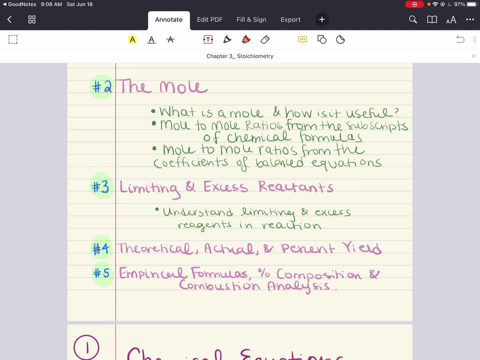 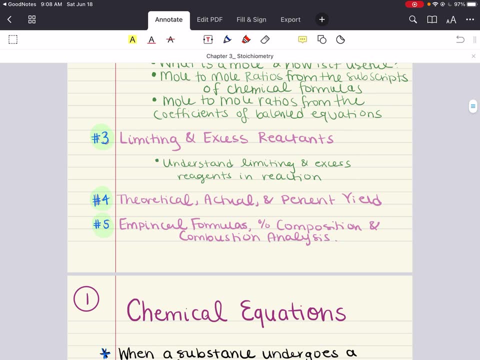 excess reactants and how to find the limiting reagent or the excess reagent, And the last two topics will be really useful for you to know in your lab courses. These topics are relating to theoretical, actual and percent yield, as well as empirical formulas. 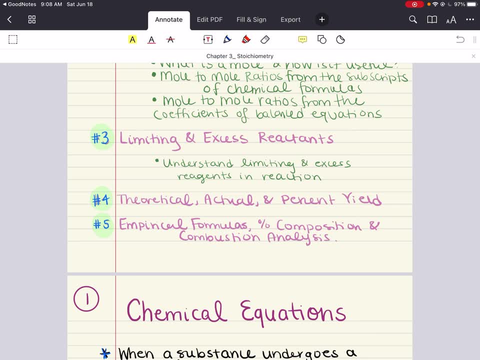 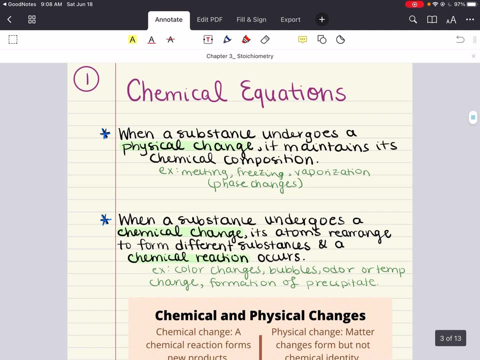 percent yield and percent yield. So let's get started. Composition and combustion analysis. So let's go ahead and start with our first topic and let's talk about chemical equations Now. chemistry attempts to understand many of the changes that occur around us. Some of the changes that we encounter can be classified as physical changes. 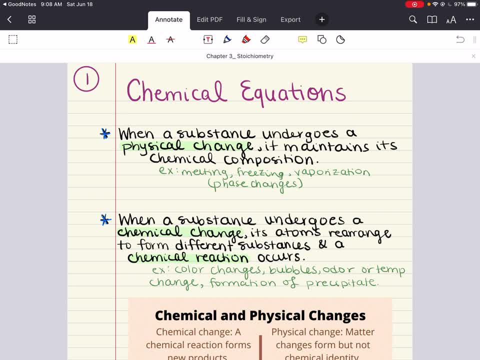 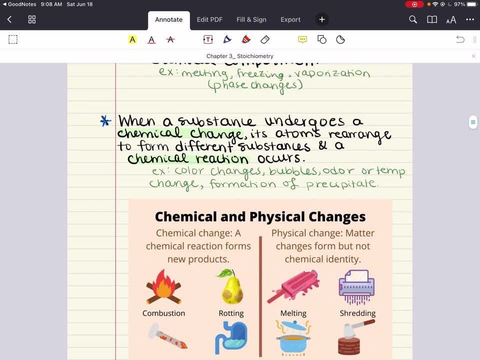 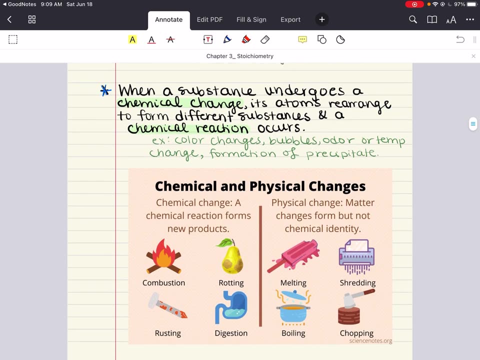 and some can be classified as chemical changes. Now, a substance that undergoes a physical change is going to maintain its chemical composition. All right, So its chemical composition is not going to change when it goes through physical changes. A good example of this: 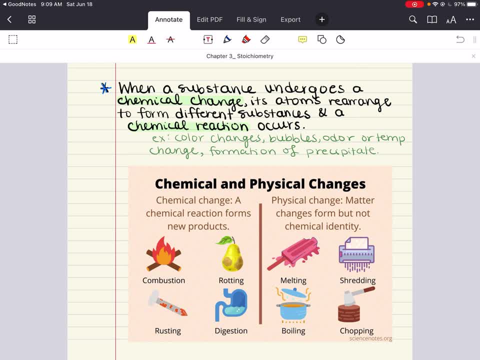 is phase changes. When water is frozen to make ice or when it vaporizes, it's still water. It's still H2O. It's simply taking another phase. All right, The chemical composition is going to maintain its chemical composition. for water, whether it's gas, liquid or solid, is still H2O. Now, when a 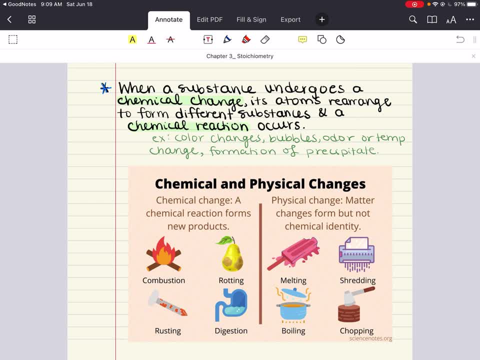 substance undergoes chemical change, all right. it does not maintain its chemical composition. Its atoms rearrange to form different substances. Things that help you indicate that a chemical change has occurred include color changes, bubbles, odor or temperature change and a formation of. 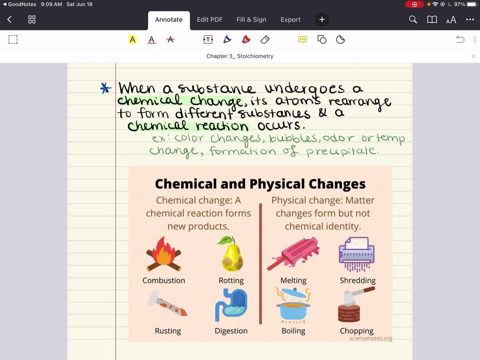 precipitate. Those are a few of the things that can happen when a substance undergoes a chemical reaction. All right, So phase changes are going to be a few things that help you identify when a chemical reaction has taken place, And this diagram here does a really nice job of giving. 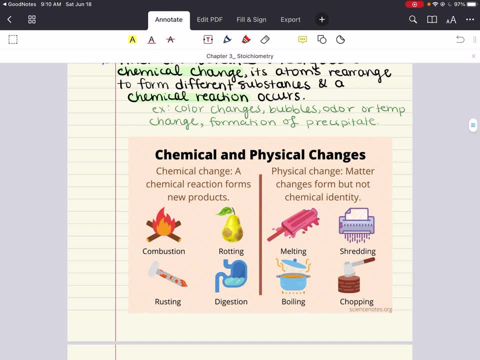 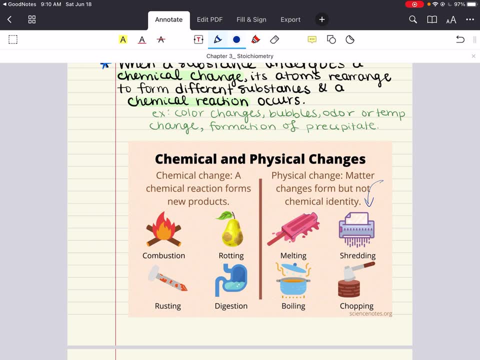 you examples of things that constitute physical changes. All right Things like melting, boiling, chopping wood- It's still wood, It's just now. instead of having one piece, you might have two or four Shredding. it's still paper, but now you just have little slits of it instead of an. 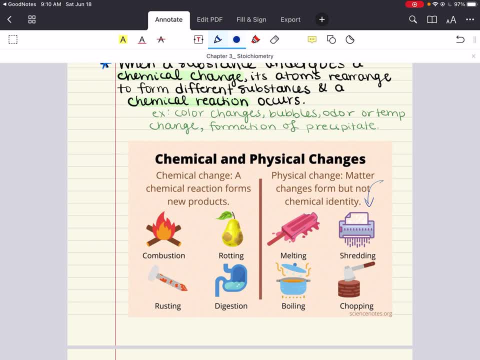 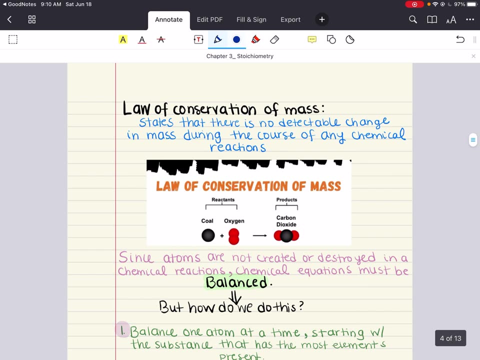 eight, by 11 or whatever, Whereas chemical changes include things like combustion, digestion, rusting- Those are all things that result in change in chemical composition. Now, an important thing to consider, in regards to both physical and chemical reactions, is that, regardless, the law of conservation of mass will hold. This law states that there is no detectable 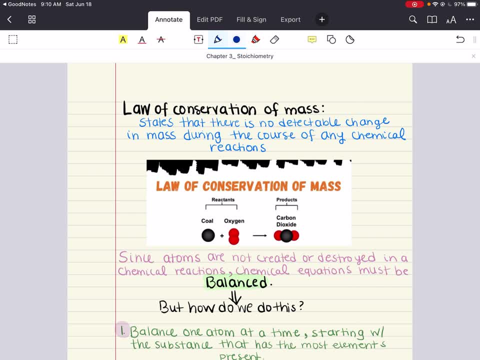 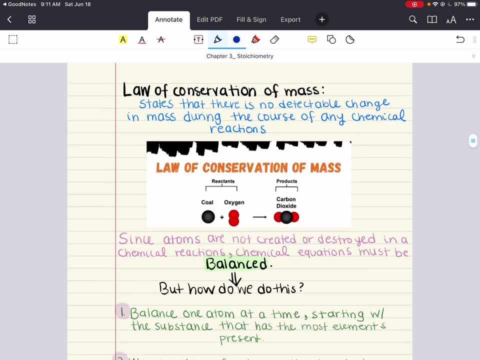 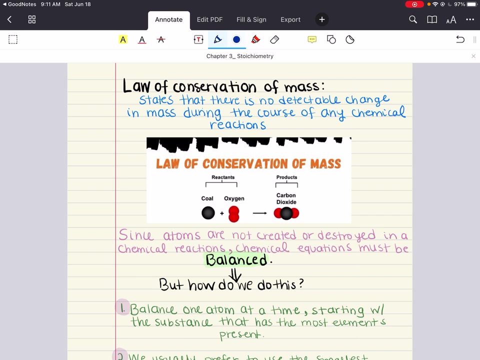 changes in mass. during the course of any chemical reaction, Atoms are neither created or destroyed. They simply rearrange To form new substance. Now, because of this, chemical equations must be balanced to assure that the atoms and the quantity of each in the reactants match up with the atoms and the quantity. 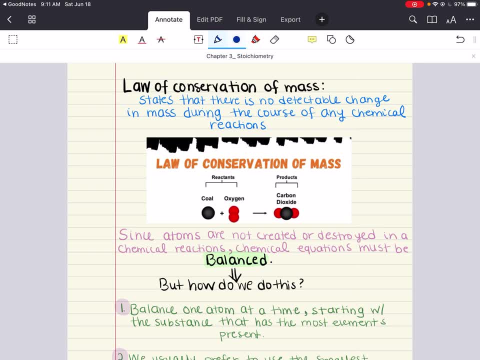 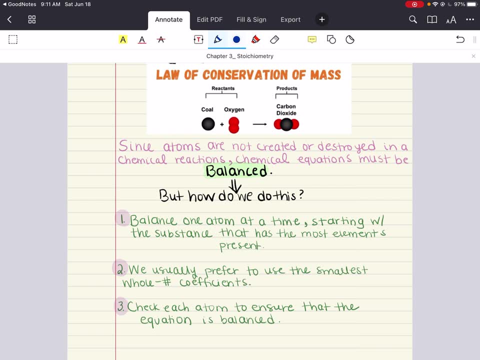 of each in the product. So if there's a total of six oxygens in the reactants, there needs to be six total oxygen atoms In the products. and this balancing of chemical reactions is done by placing coefficients in front of the formulas to indicate the relative amount of reactants and the relative amount of products. 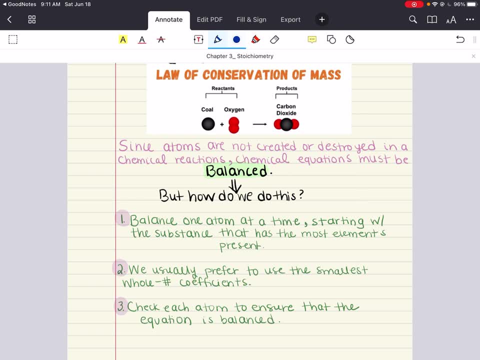 Now you might be asking: well, how the hell do I balance an equation? Here are three steps that are going to be important to keep in mind when we tackle some practice problems here in just one second. All right, These are good things to do. 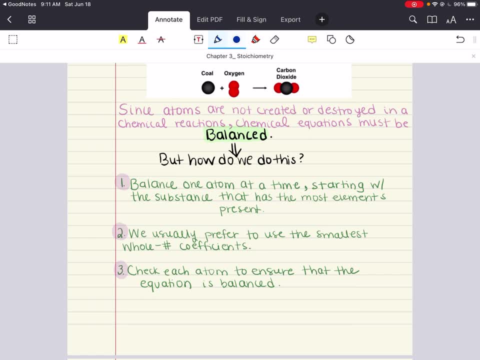 To ask yourself and to follow as you are balancing chemical equations. One balance, one atom at a time, starting with the substance that has the most elements present. Two: we usually prefer to use the smallest whole number coefficients. So no fractions, Try to no fractions, Try to avoid those. Check each atom to ensure at the end that the equation. 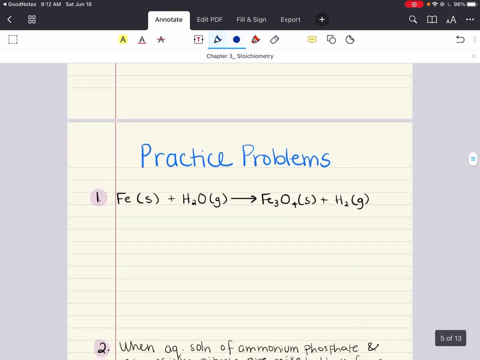 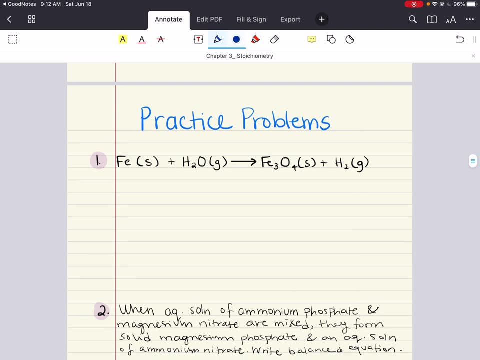 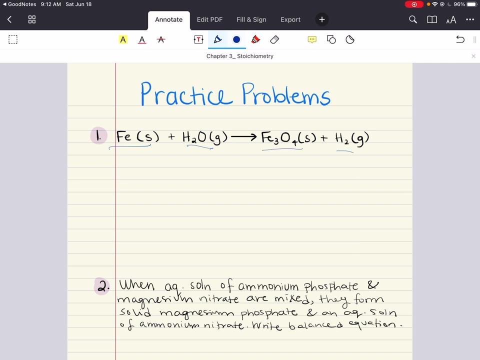 is indeed balanced, All right. So those are easy to say, but let's see this in action with a few practice problems, All right. So here we're starting off. One: we have iron, water, iron oxide and H2, hydrogen gas- All. 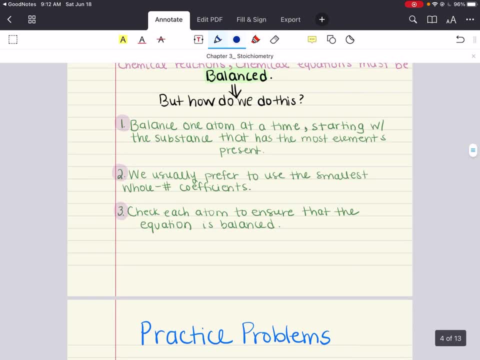 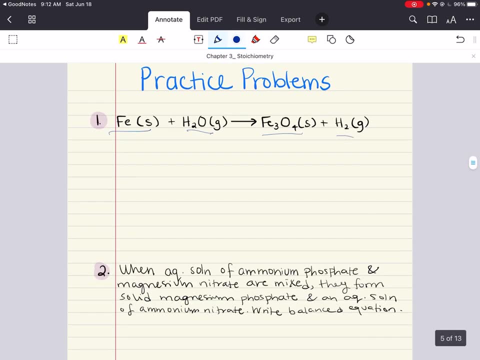 right, So we're going to balance it. And remember the first rule here: balance one atom at a time, starting with the substance that has the most elements present. All right, So that means we want to start off with one atom at a time. So we're going to start off with one atom at a time. 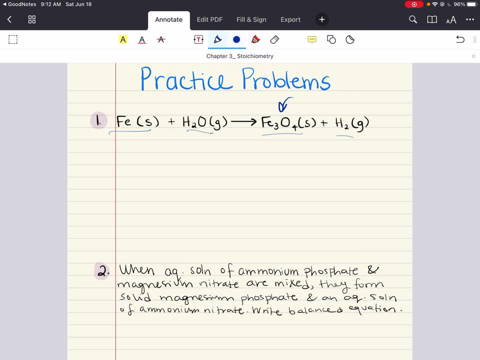 So we're going to start over here. All right, It's a good place for us to start, All right. And now we can observe here: All right, We have three irons in the product. All right, Now let's look. 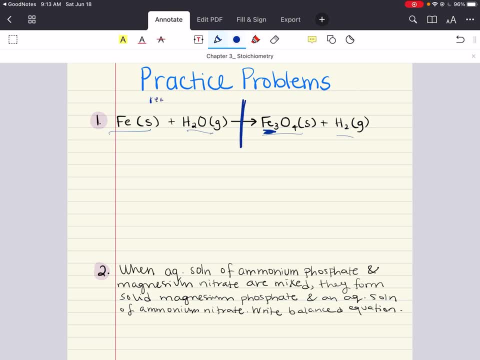 at our reactants. Remember this divide, this arrow divides reactants. These are all our reactants, our starting materials from our product. All right, We decided that this has the most elements present, So we're going to start by looking at that and trying to balance, going from there. 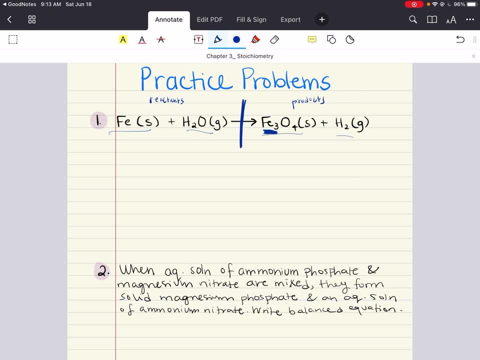 So we look at our iron, We have three irons in our product side total. If we look at our reactant side, there's only one iron. We want to get those to match up. So what are we going to do? We're. 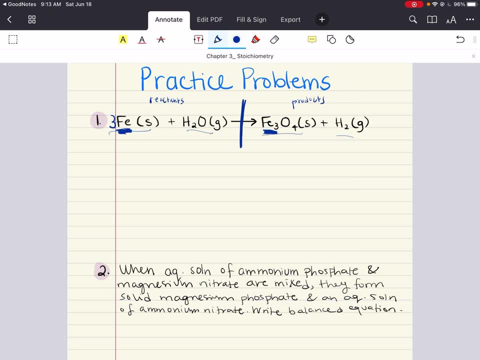 going to add a three coefficient in front of that iron. Okay, So so far all right. what we've done is we've matched the iron in the products with the iron from the reactants- Beautiful. Now let's look at this oxygen. There's four oxygens in our products. Let's look at our reactants. 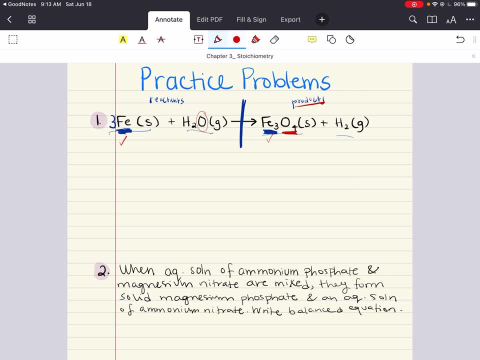 We only have one. All right, We only have one oxygen here, So we're going to try to balance that. What are we going to do? We're going to add a four coefficient in front of the whole water, All right. What this means is that now we actually have four total oxygens on the reactant side. 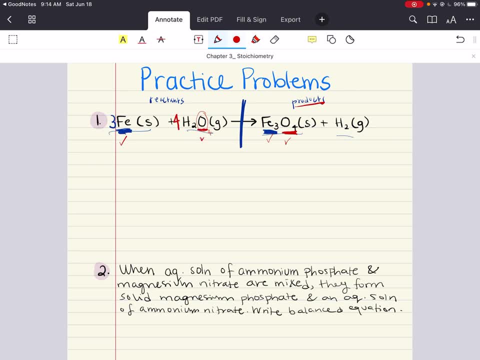 All right. So now we've matched the oxygens on both sides, All right. What do we have less left? We have hydrogen, All right. We have two hydrogens on the product side and we have eight hydrogens on the reactant side- All right. So we need to get those to match. 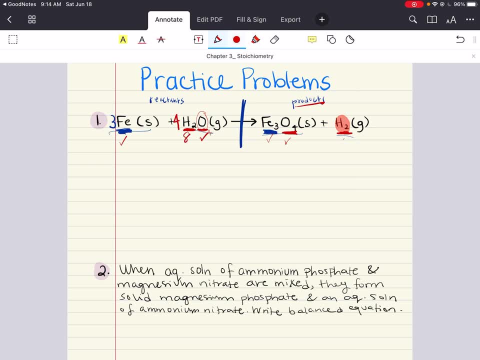 We have eight hydrogens here. We have only two here. So we're going to have to add a four coefficient here to get this to be balanced. And now we've balanced our last atoms. All right, Now all the number of iron, hydrogen and oxygen on the reactant side matches up with the 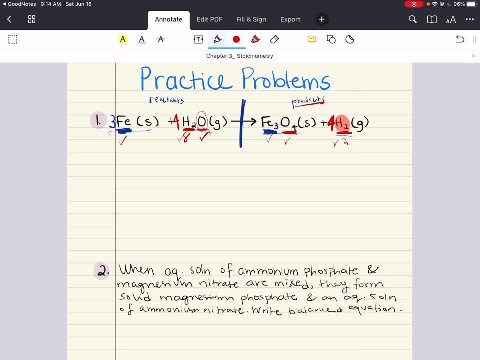 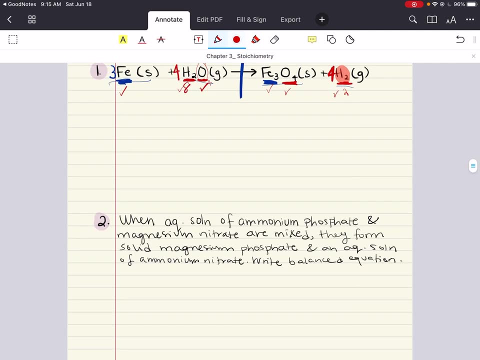 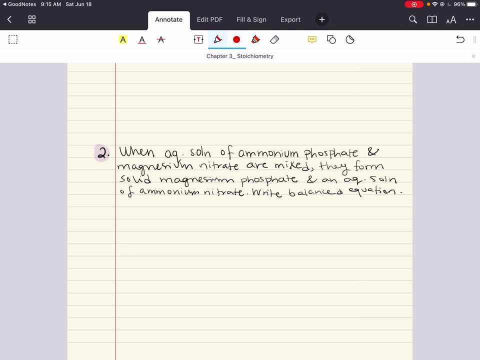 number of iron, oxygen and hydrogen atoms in the product side. All right, Fantastic. So that's one way that we can approach this. All right, Let's do another practice problem. Really, you only get good at balancing equations as you do more, because it's just a matter of observing. 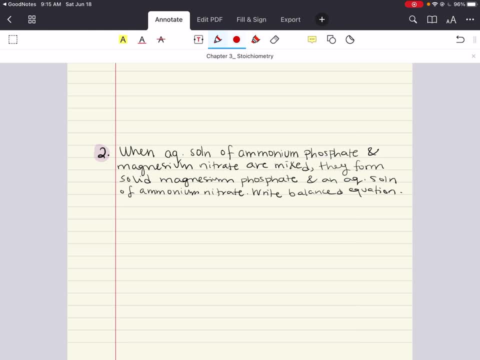 enough of these examples to get the hang of it really quickly. Let's read this next problem. When aqueous solution of ammonium phosphate and magnesium nitrate are mixed, they form solid magnesium phosphate and an aqueous solution of ammonium nitrate Write the balanced equation Fantastic. Now this is a great problem because 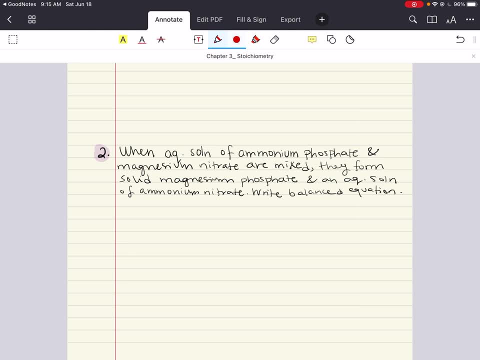 one: it requires you to remember all our naming rules from chapter two, The naming rules I told you to practice intensely, repeatedly throughout the course of general chemistry, always because you're going to end up learning other topics and somehow you're going to get problems. 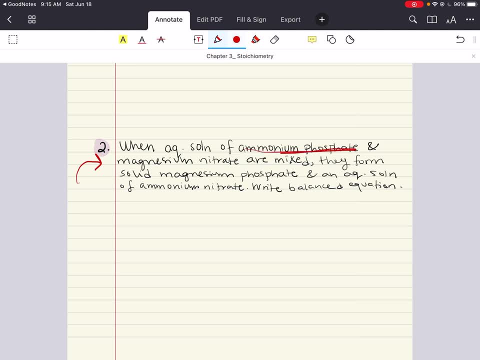 regarding balanced equations, where you still need a double check if you remember how to name molecules, just so you can do the problem appropriately. All right, So ammonium, NH4, phosphate, PO4 with a 3 minus That 3 goes down here. All right, So this is ammonium phosphate plus magnesium and magnesium. 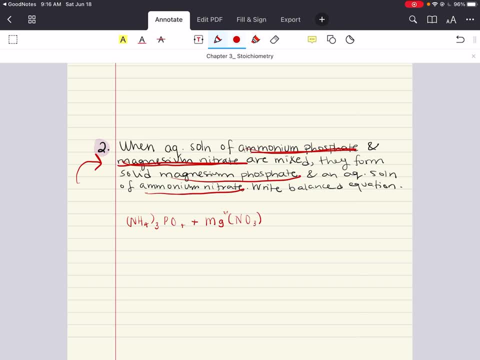 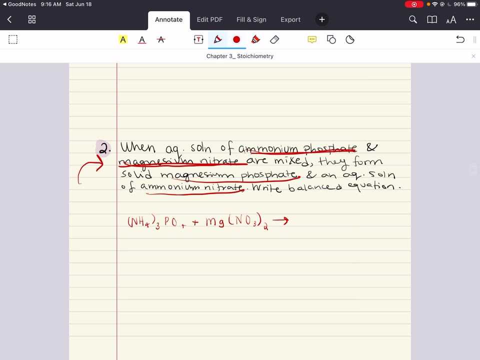 with a 2 plus charge, nitrate NO3, 2.. All right, That's magnesium nitrate for us. What does it form? Oh well, it forms magnesium phosphate. All right, So let's write that down: Magnesium phosphate, PO4 2 and. 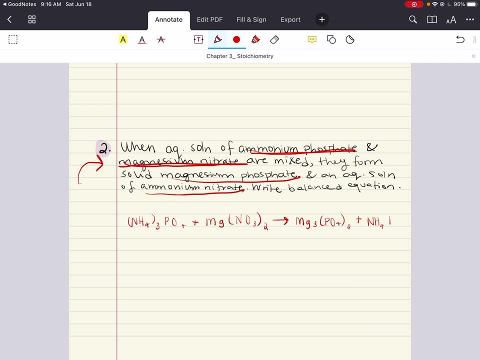 ammonium nitrate, NH4.. All right, Fantastic. So hopefully you've got the naming down, that it makes sense how we wrote out each one of these names. If not, go back to my chapter two video and work through it one more time, especially the naming section, And always remember: practice, practice, practice. Cool beans. 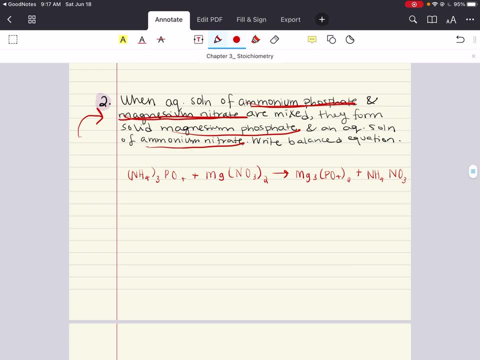 So we've written down our reaction here. Okay, Now we're going to begin balancing one atom at a time, All right, Starting with the substance that has the most elements present Now, here specifically. All right, And this is the reason why I wanted to do this practice problem. All right, There's an easier. 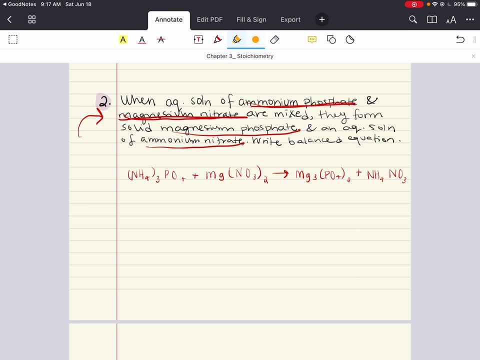 way to approach this particular reaction. All right, What you notice is that you have in the reactants and products that certain ions were exchanged but not altered. All right, What do I mean by that? Ammonium here in the reactants. ammonium here. 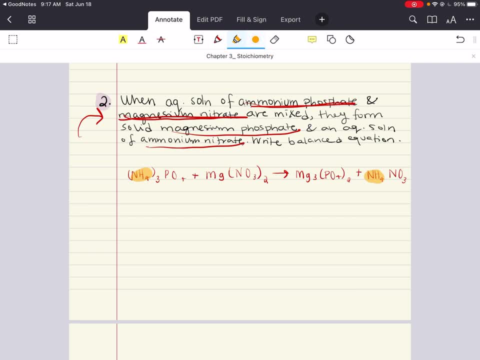 all right In the product, Okay. Nitrate in the reactants, nitrates in the products, phosphate, phosphate, All right. So you see that we're kind of more so looking at ions being mixed and exchanged more than anything else. All right, So in that case it's going to be easier to balance. 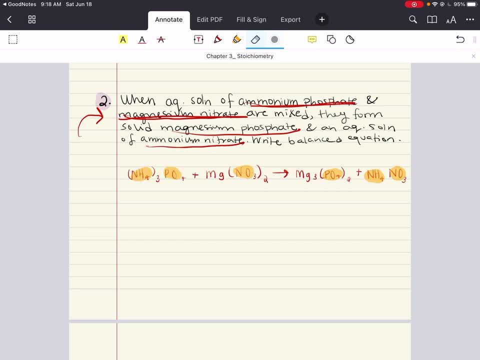 ions. oops, it's going to be easier to balance ions not changed. What I'm going to do is I'm just going to pressure this little piece though, This little little bit here. so now it's going topro这点 j то là快看正是这样 melody nòa steps. before I get that, take datuda Cryo nòa fataa. 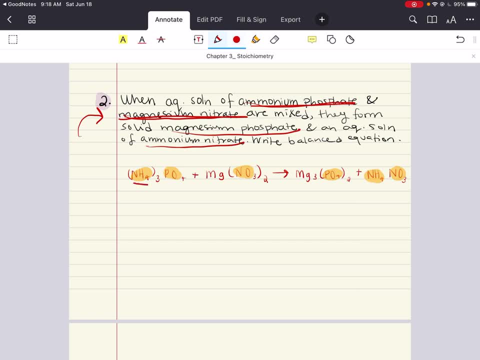 monster Drama, Iriom, not atoms. And so we're going to begin here with ammonium. All right, Again, we're going to draw this arrow, so we know this is our reactants divided from our products. We're starting here with ammonium. All right, How many ammoniums do we have on the reactants? Three of them. 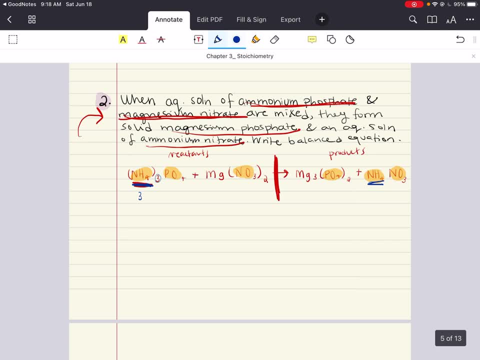 All right. And on our product side we only have one: All right. So we're going to add a three coefficient here to get these to match up. Check, Check, All right, Fantastic, All right. So now we're going to attempt to balance the next one, Phosphate. All right, We're going to attempt. 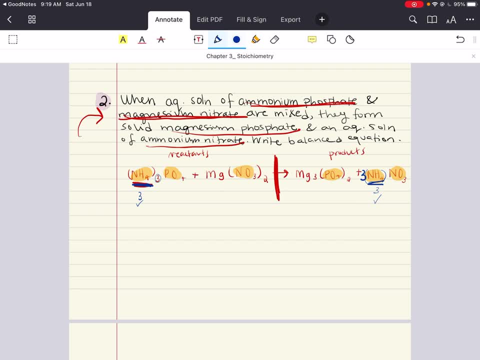 to balance phosphate. What we discover is that we need a coefficient. All right, We have a phosphate, one phosphate here, and we have two over here. Okay, We have one over here. I'm going to use a different color: purple. one phosphate in our reactants, two in our products. What does? 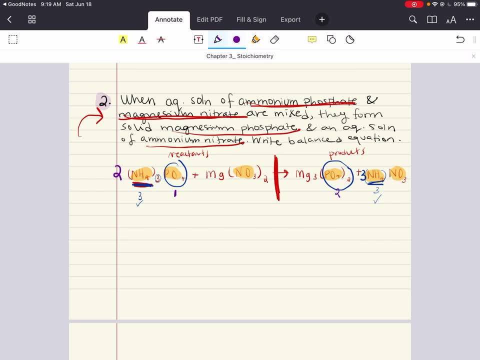 that mean We're going to have to put a two right here at the beginning- All right- Of this term, so that we can have now two phosphates here, two phosphates here, Check, Check. All right, We're going to pause. This means that we have to go back and reevaluate this, because now we've put a new. 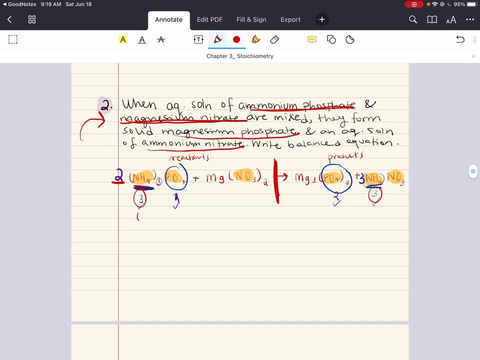 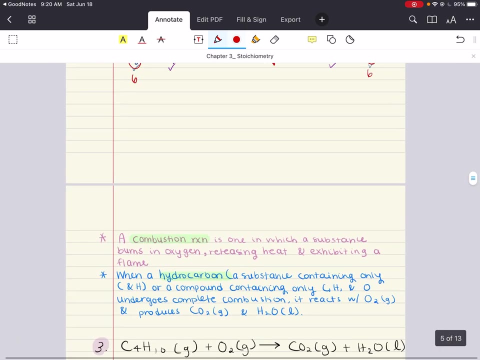 coefficient in front And that means on the reactant side now we actually have six ammonia. All right, And if we remove this three right here from our other one, that means we're going to want to put six in front of here so that we can have six on both sides. So we have to reevaluate. 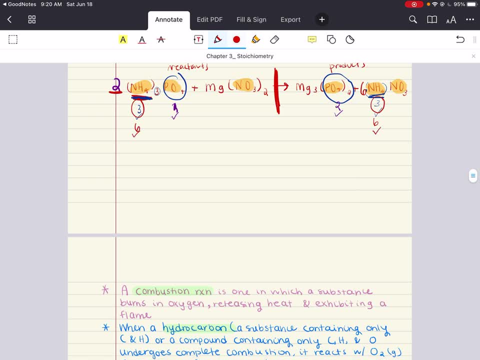 what we did in our first step, And now they're rebalanced again. So that's good, All right. Now we want to move on to magnesium. All right, Here we have one magnesium, Here we have three, All right, And so, as a balancing act, we're going to put three here. So now we have three. 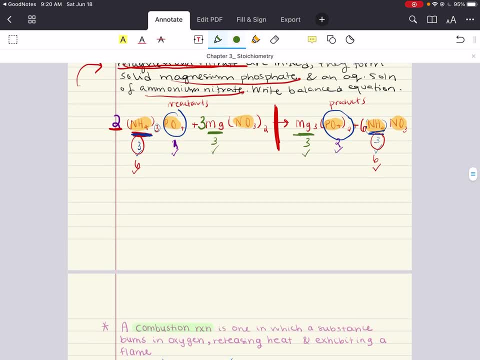 magnesium in the reactants, three magnesium in the products, Perfect. And then, last but not least, we're going to look at our nitrate. All right, On the reactants, we have three times the two that we have there, So we have a total of six nitrates that I'm going to do in black here, All right. And 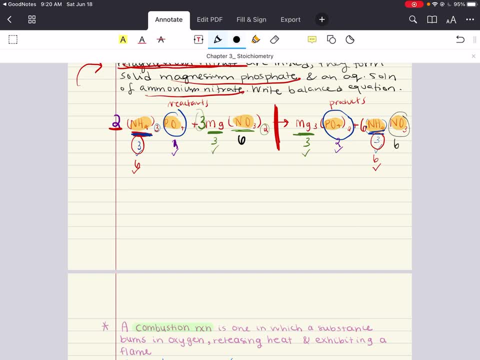 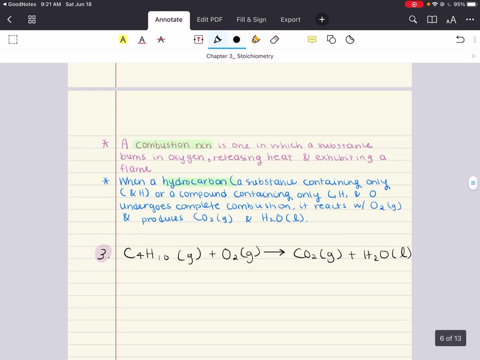 if we look on this side, we already have six nitrates. They're already balanced and we are. equation is now balanced, Fantastic, All right. Well, one more quick note here. in regards to this topic of balancing equations, I want to define a term, All right Now, in the realm of reactions, 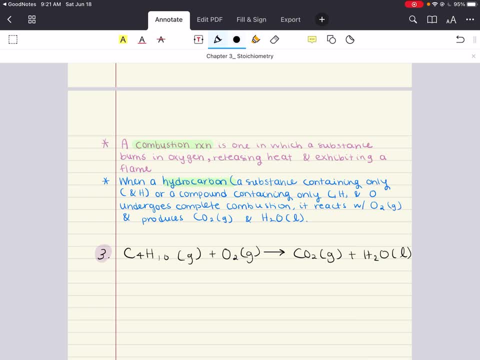 there is one that is important for us to know in general chemistry, and that is the combustion reaction. All right, This term is used to describe reactions where something burns in oxygen gas. It is going to be characterized by the release of heat, All right, So that's important. 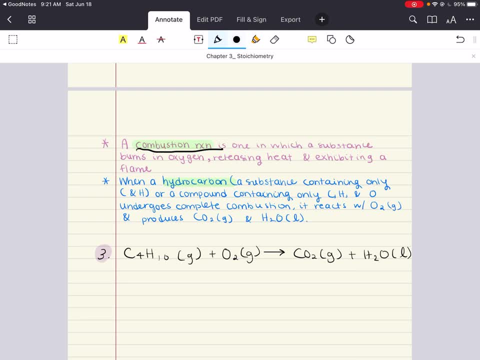 to know. It's going to be characterized by the release of heat and presence of a flame. We will see the combustion reactions in general. We're going to see combustion reactions specifically the ones that are just looking for a block, But we also see the response of the body. The body is. 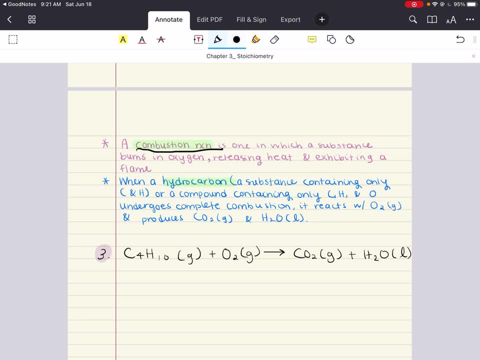 going to be focussed on the combustion reactions And that's going to be the reaction of carbon atoms. So if we look at the formula and we take a look at the reaction- reaction that we're going to see in this example, the reaction- reaction to carbon atoms- is a reaction. 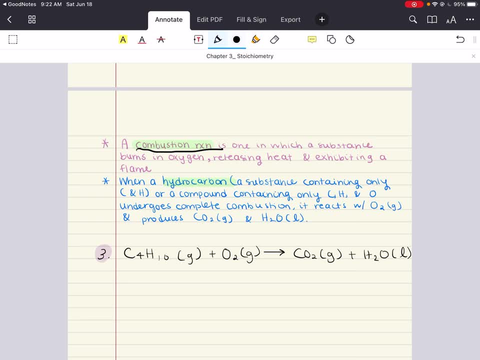 reaction that is going to be based off of the absorption reaction. So if you look at the formula, where there is just carbons and hydrogens, that molecule is referred to as a hydrocarbon. We're going to see combustion reactions of hydrocarbons. Now, when a hydrocarbon undergoes 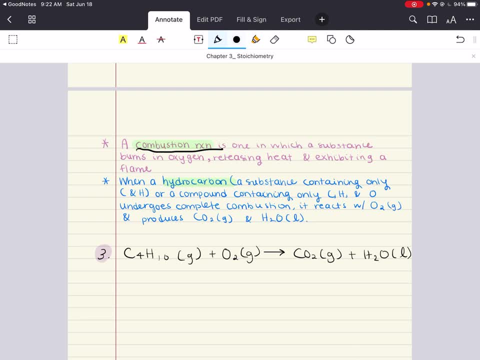 complete combustion in oxygen gas, the products are always going to be be carbon dioxide and water. Now, this practice problem that we're going to do right here is a good example to identify these terms. Here's our hydrocarbon. Notice it's only carbons and 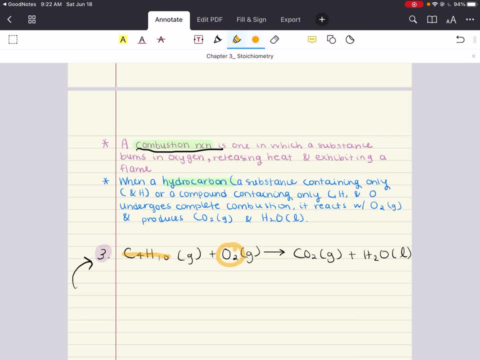 hydrogens. Here is our oxygen gas, Now the products of a hydrocarbon, and oxygen gas is a combustion reaction, and so we're going to form carbon dioxide and water as our product. All right, fantastic. So let's balance this equation now that we know what a hydrocarbon is. 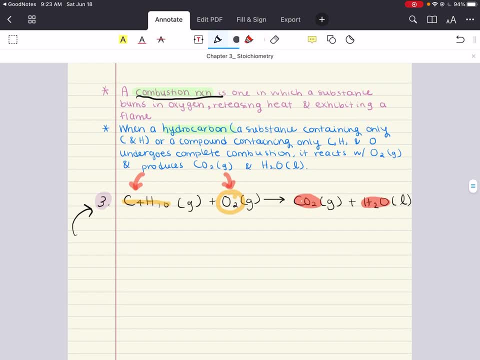 All right, we're going to start off with our carbon atom here. All right, we're going to look at our carbon atom. We're going to divide. Here's our reactants, Here are our products. All right, we're going to look over here. We have four carbons on this side. 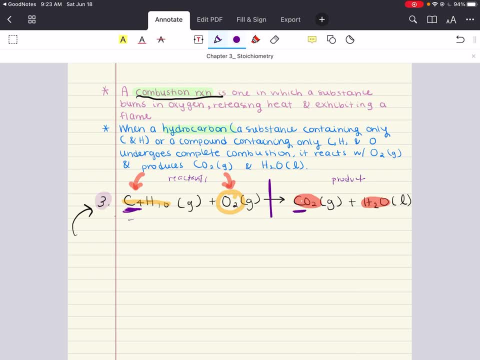 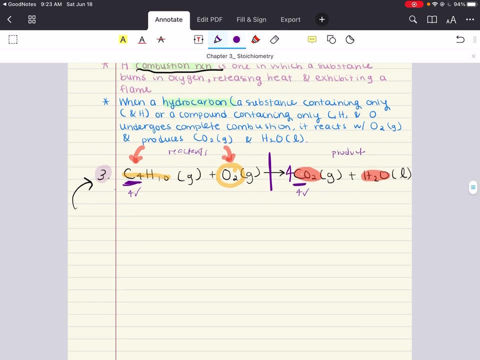 but we only have one carbon on this side. So to get them to balance, we're going to put a four in front of this carbon dioxide. So now we have four carbons on one side, on the reactant side, and four carbons on the product side. Fantastic, All right, let's move on to our next atoms. 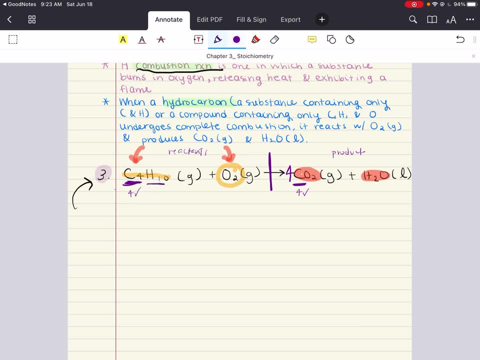 All right. now we want to look at our hydrogens. All right, we have a carbon atom. We have 10 hydrogens on this side. all right, but only two on this side, So to get that to be 10,. 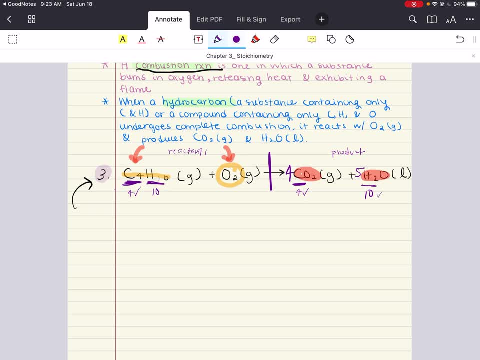 we're going to put a five. Five times two, that's 10.. Now we have 10 hydrogens on both sides. All right, next up is going to be our oxygen. On our reactant side, we only have two oxygens. 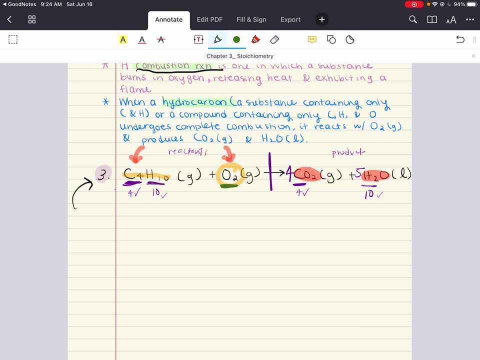 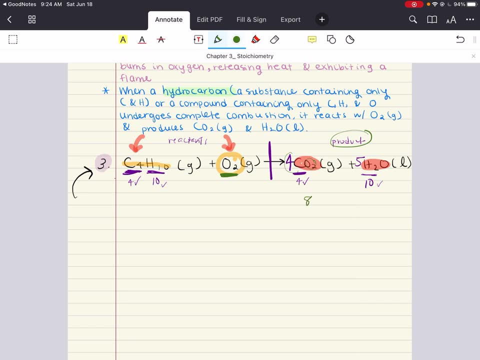 All right, that's good to know. On our product side, however, we have, all right, four times two- Eight oxygens here and five times one and five right here. All right, perfect, All right. so then that means we have a total of 13 oxygens. All right, we have 13 oxygens. 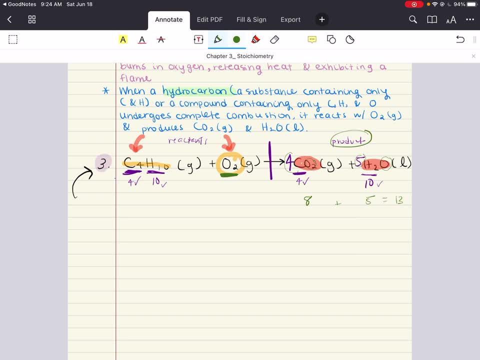 on the product side. Now to balance the number of oxygen atoms on the reactant side, we're going to do something that is, in the end, going to be illegal, But we're going to fix it up really quickly. All right, we have a total of 13 oxygens on the 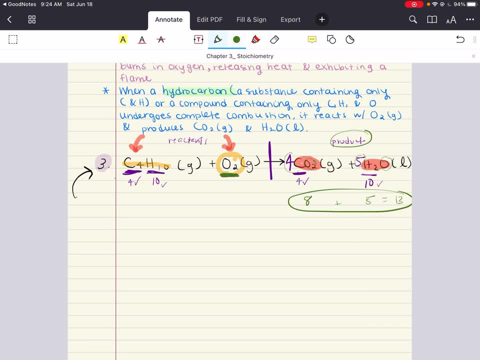 product side, All right, and on this reactant side, we only have two. What we're going to do right here is we're going to multiply it by a fraction of 13 over two. All right, 13 over two times two is going to be 13.. But at the end of this, all this isn't going to be correct. 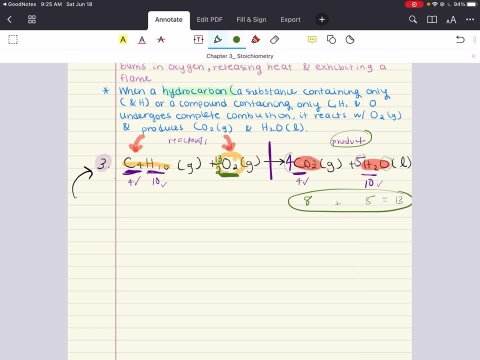 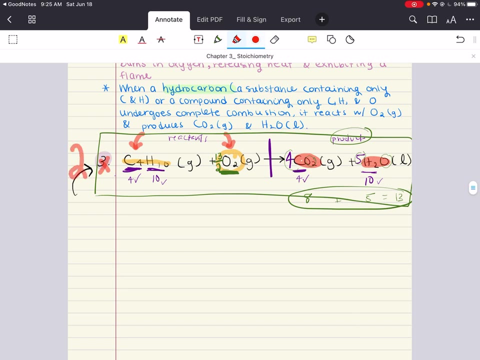 because we can't have fractions. all right when we're balancing equations. So how are we going to fix this whole equation now that we have a fraction in our oxygens for our oxygen gas? Well, we're going to multiply the whole thing by two. What that does is it's 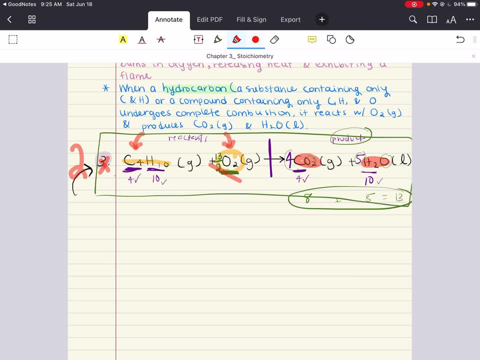 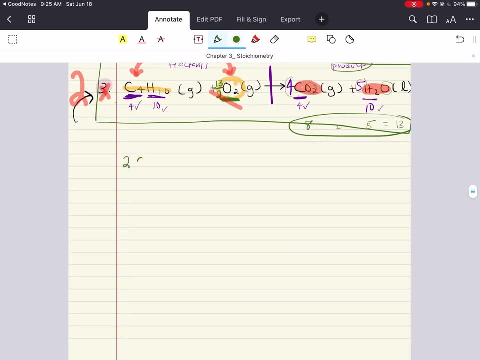 going to get rid of the two in the denominators and it's going to let us reach our final balanced equation. So if we multiply everything by two, then our reaction is going to be two C4H10 plus 13 C4H10.. 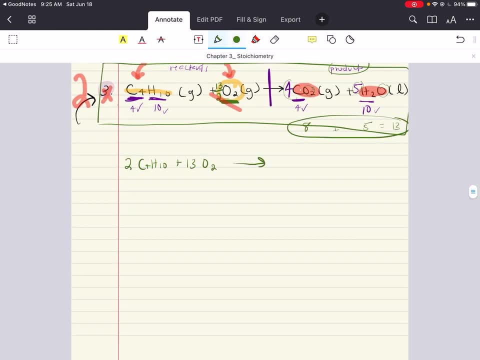 O2 for the reactants And then for the product side. remember we're multiplying by two, So eight CO2 plus 10H2O And this is our final balanced equation. All the atoms are balanced. You can double check. Everything matches up. The equation is correct, Fantastic. So that is kind of like a. 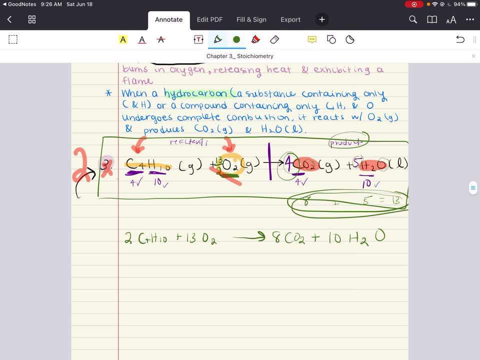 little hack on how to balance equations when it comes down to something like this, where it might be hard for you to then go and readjust. So let's go ahead and do that. So let's go ahead and do that. So let's go ahead and readjust every single number on your own. Put a fraction, All right, And 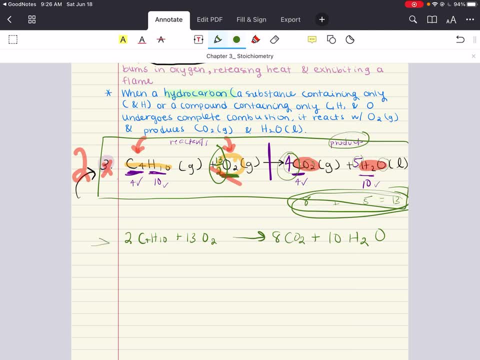 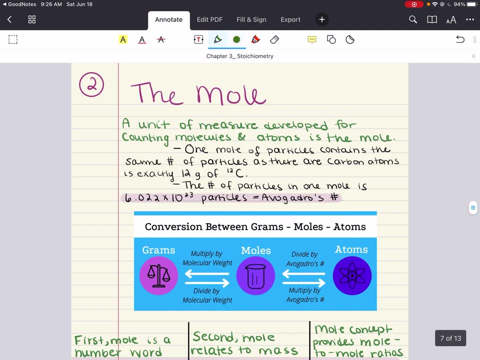 then multiply through to get rid of the fraction, And then double check to make sure everything is balanced. Fantastic. Now on to our second topic, the mole. In order to simplify calculations, a unit of measure has been developed for counting molecules and atoms, And this unit is known as. 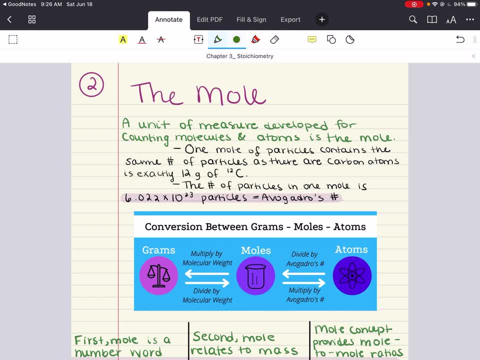 the mole. A mole is defined such that one mole of particles contains the number of particles, as there are carbon atoms in exactly 12 grams of carbon-12.. All right, So let me rephrase that in a way that we're all going to understand: The number of particles in one mole is 6.022 times 10 to the 23.. All right, 6.022 times 10 to the 23.. And then we have the number of particles in one mole. And so we have: the number of particles in one mole is 6.022 times 10 to the 23.. All right, 6.022 times 10 to the 23.. 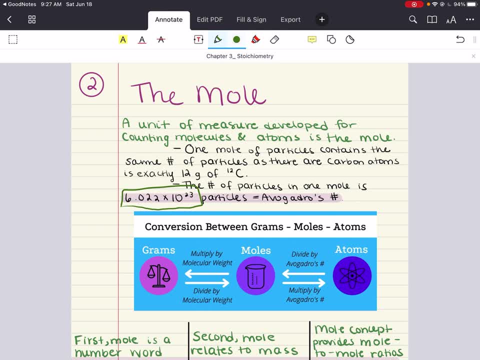 So we're going to find it. And then let's go ahead and do our next question. We're going to go ahead. and 10 to the 23 particles equals one mole. This is known as Avogadro's number. It is a unit of measurement. 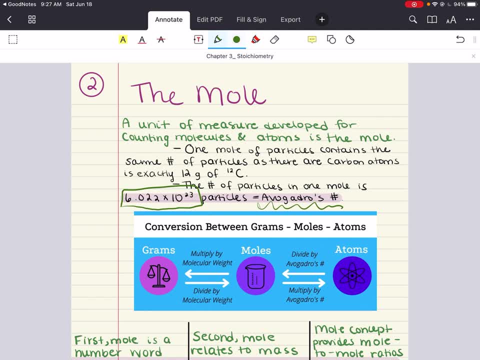 Like saying one dozen eggs. you know that that means dozen means 12.. So that means when you say one dozen eggs, that is equal, all right, to 12.. All right, it's the same thing with Avogadro's number. 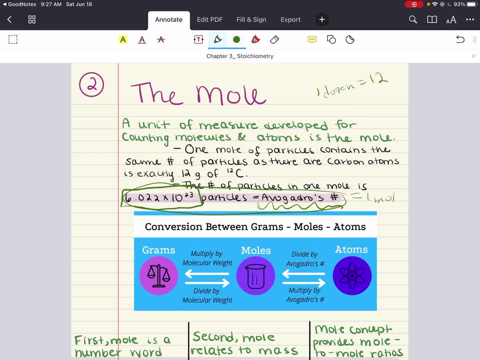 One mole is equal to Avogadro's number of particles. All right, and this is going to help us a lot in things like dimensional analysis and conversions, So we need to be able to understand this so we can take advantage of it in regards to those things. 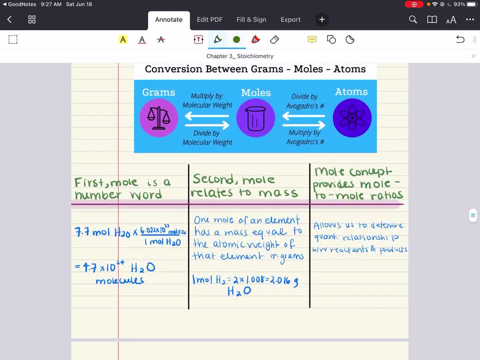 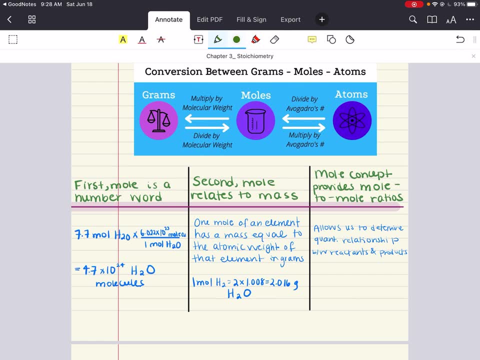 There are three important points we want to make about the mole, though, before we get to some practice problems. One: mole is a number word. okay, It can be used as a conversion factor in dimensional analysis. Two mole relates to mass. 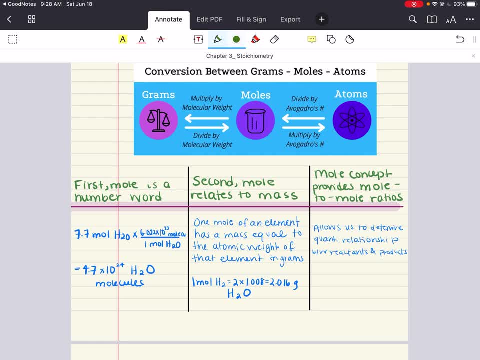 One mole of analysis, One element, has a mass equal to the atomic weight of that element expressed in grams. One mole of H2 is simply equal to 2.016 grams, which is the molecular weight of H2.. All right, simple. 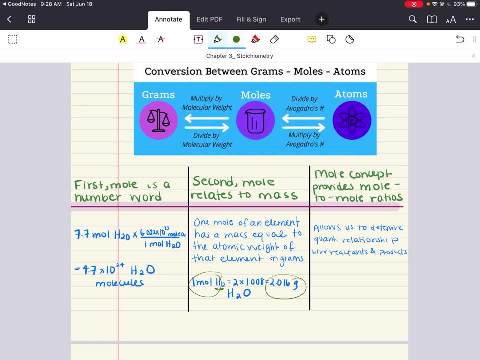 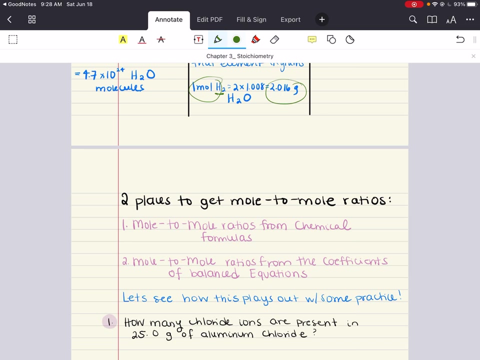 All right. three: the mole concept provides mole to mole ratios. This allows us to determine quantitative relationships between reactants and products and chemical reactions. There are two places that we're going to be able to get this mole to mole ratio: the subscript of a chemical formula, all right, and the coefficients of a balanced equation, all right. 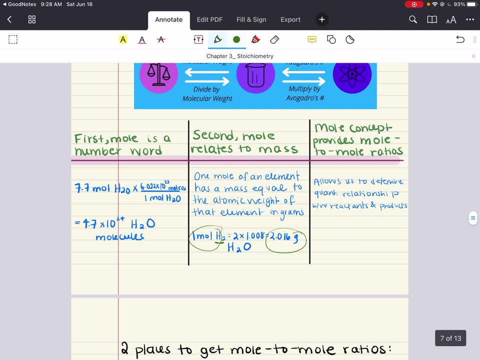 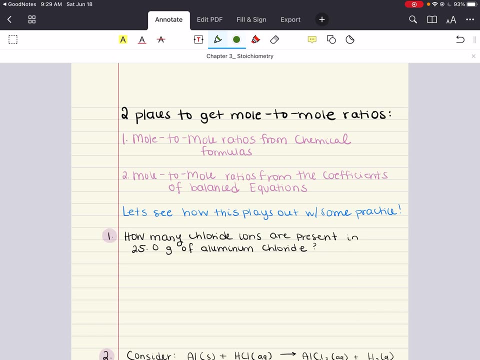 So those are important things to know. First, mole is a number word. Two, second, mole relates to mass. And three mole concepts provide mole to mole ratios that we can get from two places: chemical formulas and balanced equations. So we're going to see how this plays out, with some practice problems now. all right, 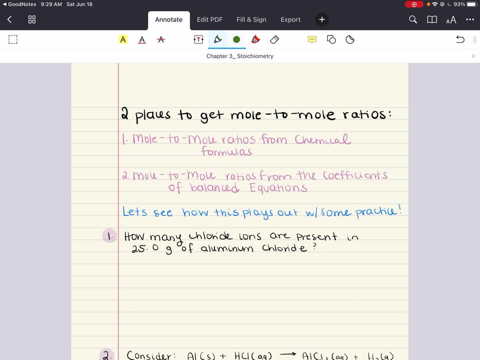 We're going to see exactly how we can take advantage of the mole. all right, to answer questions that are going to require us to do some conversions: How many chloride ions are present in 25 grams of aluminum chloride? all right, All right, so we're going to. 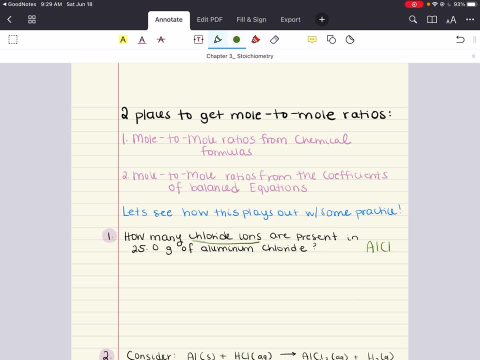 Try to answer this. Aluminum chloride. All right, how many chloride ions are present in 25 grams? So what we're going to do first is we're going to write what we want to know. What is it that we want to know? 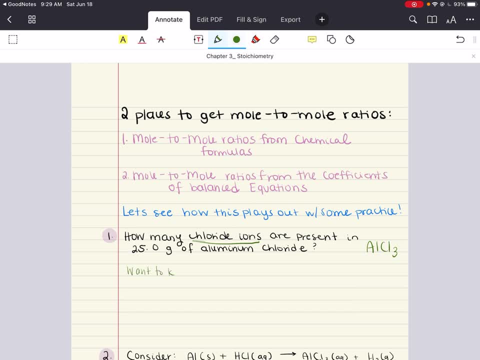 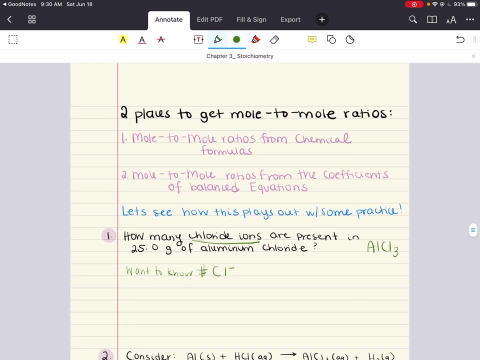 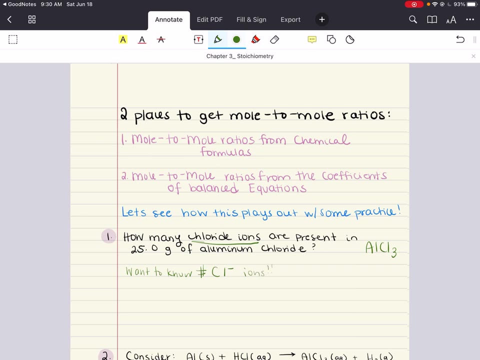 We want to know the number of chloride ions. All right, that's what we want to know. So that means we're going to start off with a given measured quantity. They gave us a given measured quantity and we're going to take advantage of it to do some conversions, some dimensional analysis, like we've done in chapter one, to go from what we have to what we want to know. 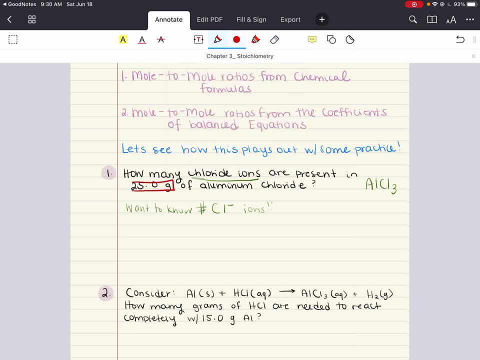 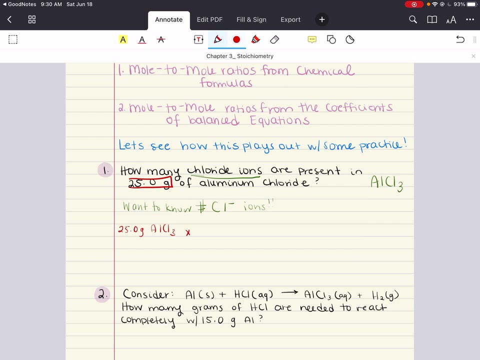 So how are we going to do this? We're going to start off with 25 grams. 25 grams of what exactly? Aluminum chloride. That's what we know, okay, Okay, So we're going to go and we're going to convert this all the way, however many steps it requires, or conversions, to get to number of chloride ions. 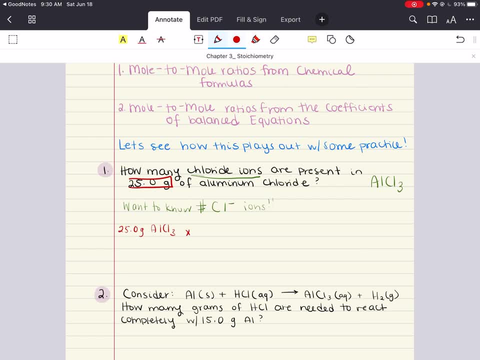 So the first thing we want to do is we can convert this gram to moles. All right, that would be a good start. Now, the molar mass of aluminum chloride. I'm just going to go ahead and give it to you, all right. 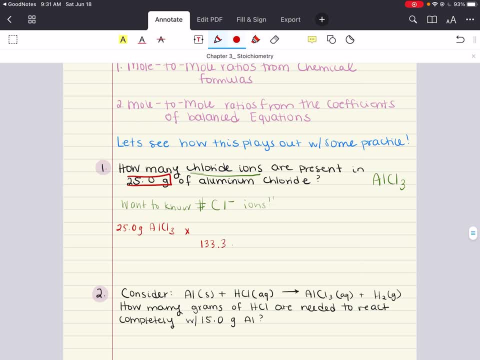 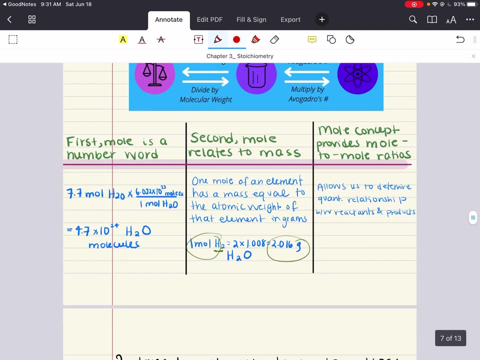 It's 133.3 grams, All right. All right, That's the mole, That's the molar mass of aluminum chloride. All right, this equals to one mole of aluminum chloride. Remember the second point: mole relates to mass. 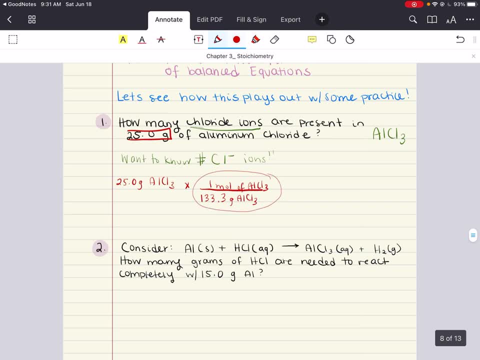 That is why we can write this: that the molar mass of aluminum chloride- 133.3 grams of aluminum chloride- is equal to one mole of aluminum chloride. All right, now next up. this is really cool. This is where we get to see, all right, how we can get. 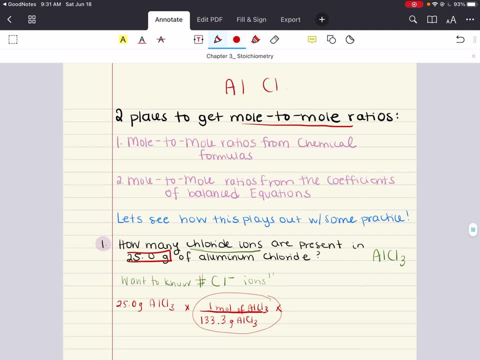 How we can get mole to mole ratios. Look at aluminum chloride. All right, this is aluminum chloride. You have one for one mole of aluminum chloride. you have three moles of chlorides. All right, You can get mole to mole ratios from chemical formulas like this. 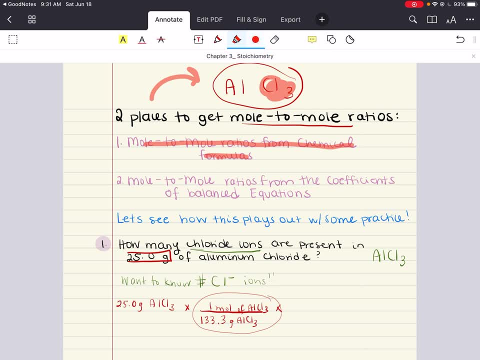 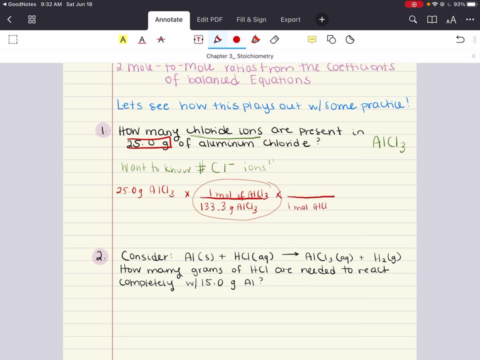 So two. one for one mole of aluminum chloride. you have three moles of chlorides. We're going to use that as a conversion here. One mole aluminum chloride Is equal to three moles of chloride ions. All right, and now for the last step, so that we can get what we want to know: number of chloride ions. 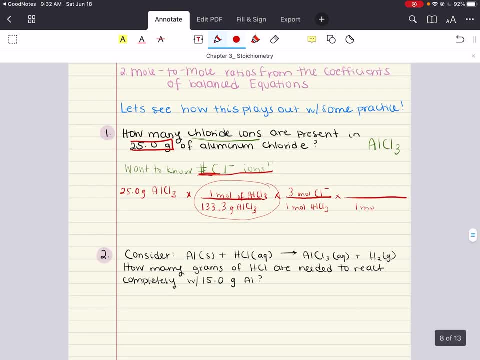 We're going to take advantage of the fact that we know one mole. all right of an element is equal to 6.22 times 10 to the 23 of that element in ions or formula units or whatever particles. All of that is synonymous. 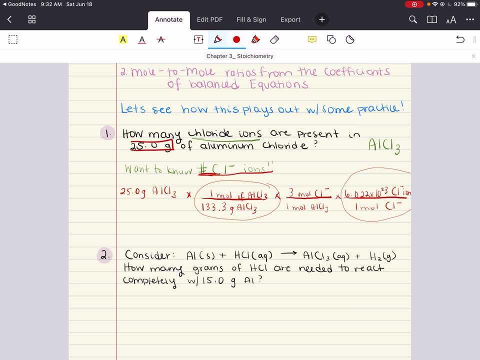 All right. So we use Avogadro's number as well as our final conversion, and that means that- look at this- everything cancels out. Grams cancels out with grams. here. Mole of aluminum chloride cancels out with a mole of aluminum chloride. 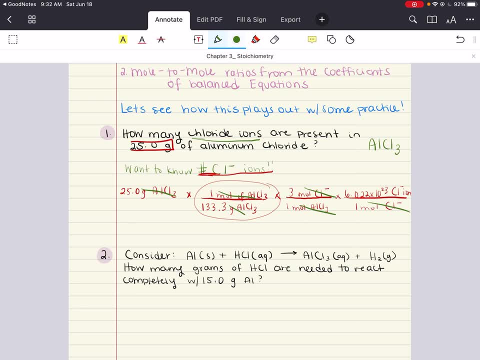 Mole of chloride cancels out with mole of chloride and we are left with number of chloride ions as our unit. So whenever we get this number by plugging it into the calculator, the unit associated with that number, which is the number of chlorides, is going to be zero. 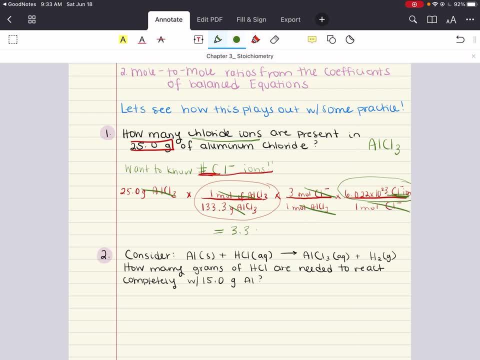 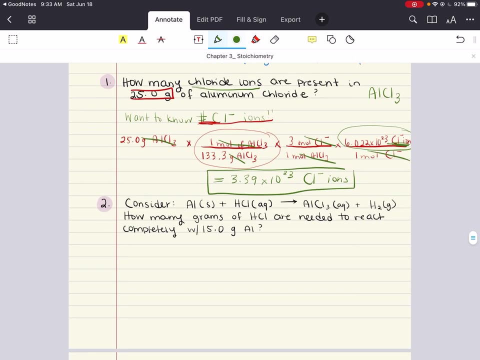 It'll always be zero. It's going to be zero number, which is 3.39 times 10 to the 23. the unit associated with it is chloride ions, and that is how you answer this question. i'm gonna leave two for you to try to figure out. let me know what you. 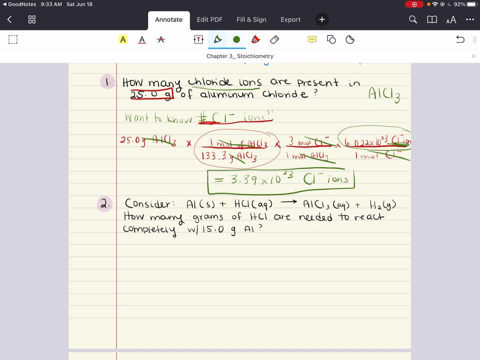 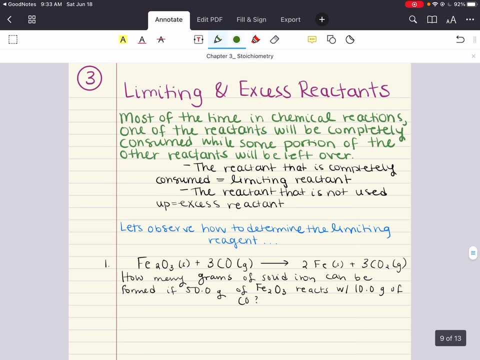 get in the comments below, all right, or if you need help and we can try to figure out together, then, but i want you to give it a shot, all right, and let me know what you get. all right now, moving on to our third topic of the chapter, we're going to be talking about limiting and excess reagents. 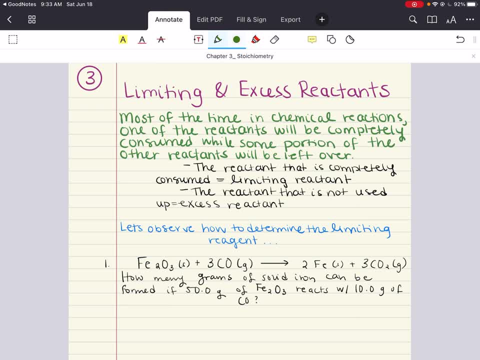 here. when chemical reactions are carried out, most of the time one of the reactants is going to be completely consumed before the other reactant. the reactant that is completely consumed in a chemical reaction is going to be the limiting reagent. all right, and the substance that's not used all up is. 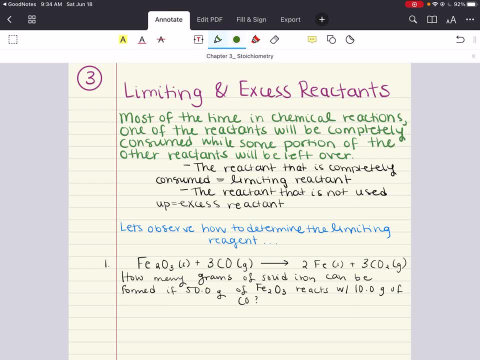 the excess reagent. all right, that makes sense, right? the one, the reactant that is completely consumed in a chemical reaction is going to be the limiting reactant, because you cannot continue with the reaction any further when one of your reactants are completely consumed up. all right, and so it's going to limit the amount of products. 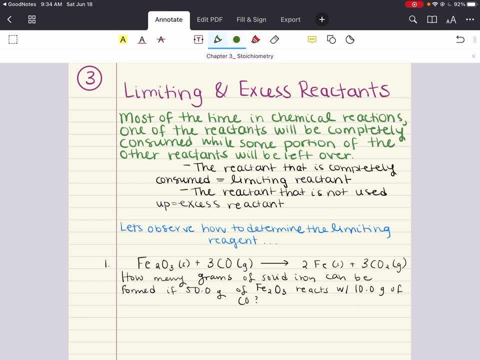 you'll be able to form because one of your required ingredients gets used up all right. so that's one way of thinking about that. but the best way to really understand how to even um assign which one of your reactants is the limiting reactant and which one is um the excess reagent, is really to do a practice problem to see how you 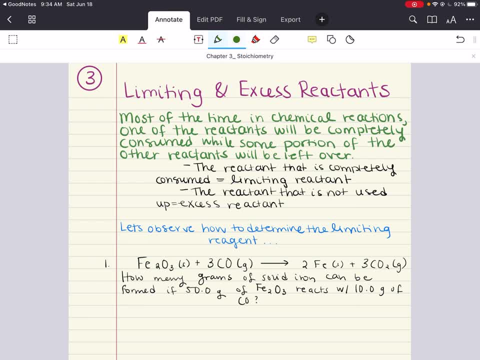 can figure out: um, what is your limiting and what is your excess reagents? so let's look at this problem here. all right, we have a reaction. here's our reaction. we were given the reaction and it's all balanced and ready for us. the question is well, how many grams, how many grams of solid iron can be formed, all right. so it's asking us how much. 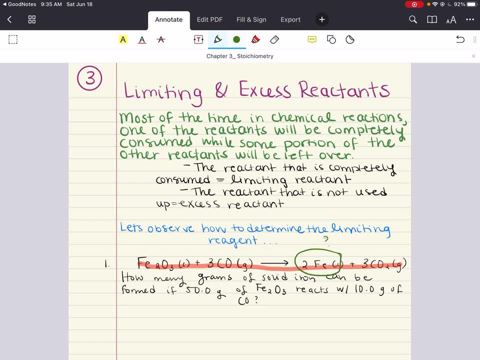 of this can be formed. if you're gonna start off with 50 grams- all right- of iron oxide and 10 grams of carbon monoxide, all right. so how much can you form of just solid iron if you have 50 grams iron oxide and 10 grams? 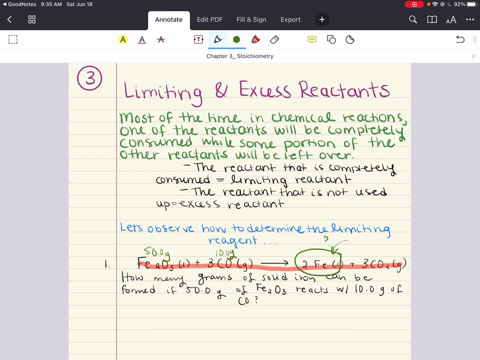 carbon monoxide, all right. so in a reaction stoichiometry problem, all right. if you are given the mass of two reactants, you're gonna have to decide which one of these is the limiting reagent. one way to do this is to say that you're going to have to decide which one of these is the 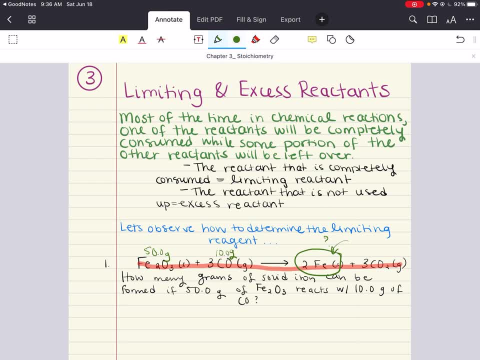 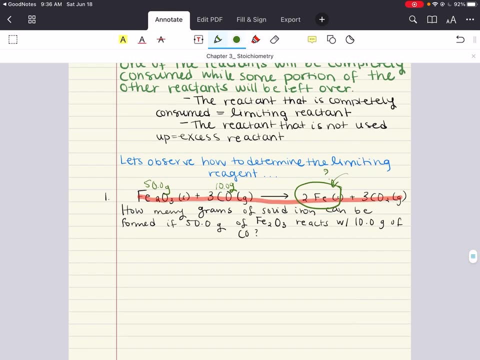 area of the product. okay, so let's go through this and do that. well, you're going to create the idea that you are on either side, all right. you decide you're gonna create the limit reagent around you. C genius, this is aprehands conference. okay, then you're gonna set up two cases, all right. 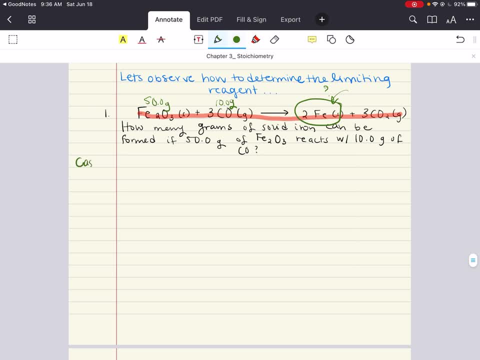 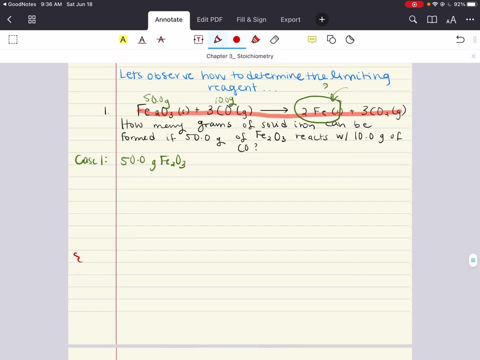 where you calculate the maximum amount of product you would get based on each reactant, then the reactant which produces the least amount of product is going to be your limiting reagent. what does that mean? what that means is you're gonna set See oxide, All right, And then you're going to set up case two here. Sorry, Case two here. 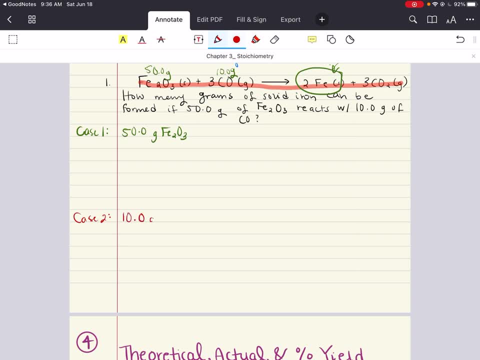 where you're going to figure out how much solid iron are you going to form from carbon monoxide, All right, And then you go through the stoichiometry of each one and see which one gives you the least amount of iron. That is going to be your limiting reagent. So 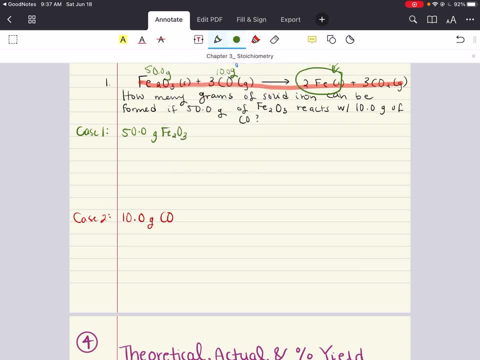 let's work these out. Let's work out case one. You're starting off with 50 grams of iron oxide. All right, We're going to do some stoichiometry here. What is we're going to take? grams, We're. 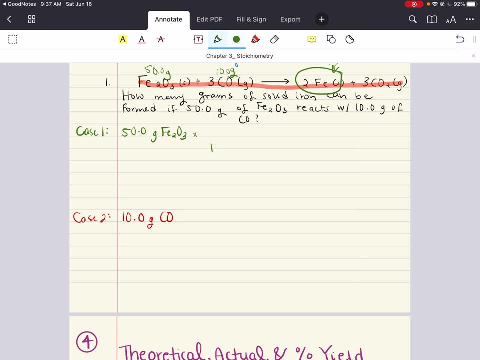 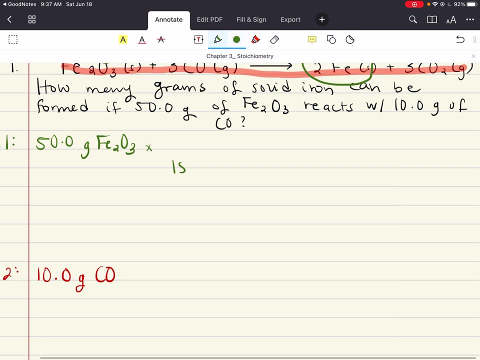 going to convert it to moles, because that's our best case here. How much? what is the molar mass of iron oxide? I'm going to give that to you. You can easily figure that out by adding up each atom together, but it's 159.7 grams iron oxide. All right, And remember our 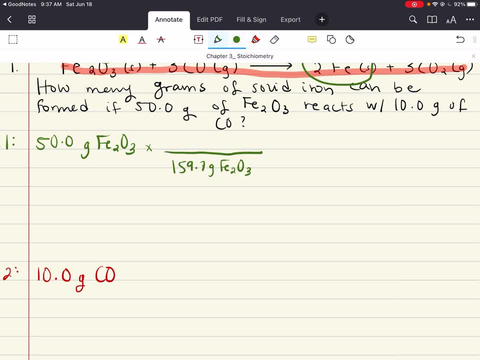 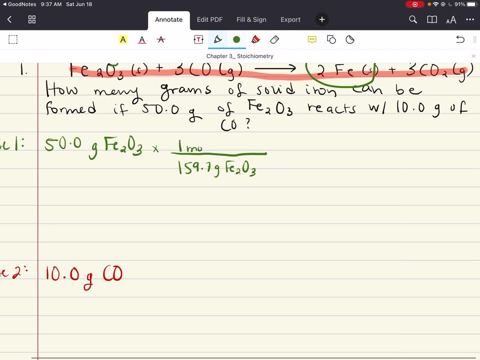 remember one of our relationships With mole. mole relates to mass, So this is the molecular mass of iron oxide. This is going to equal to one mole of iron oxide, So we're going to use this relationship here. Fantastic, Now for. 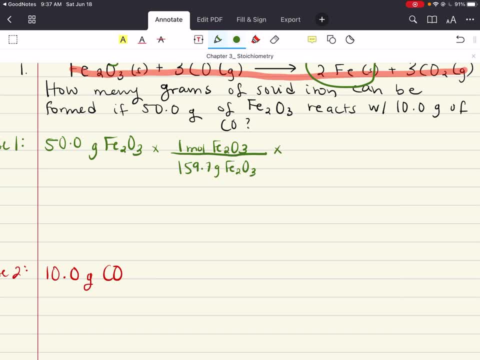 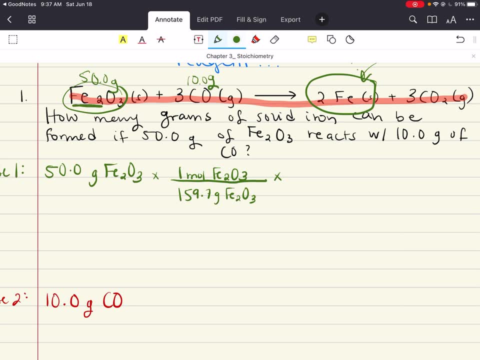 for every mole of iron oxide, right here. Okay, How many moles of iron are there? Two, All right, And that's. this is an important conversion, because we ultimately want to know how much of the solid iron oxide is there. So we're going to use this relationship here, All right, And 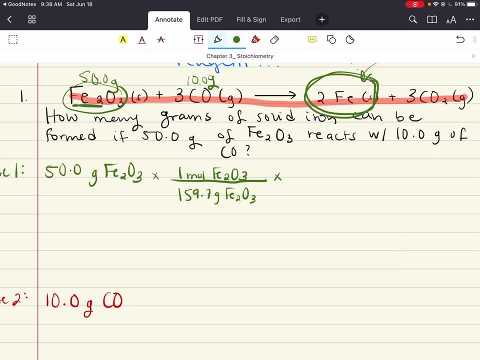 so we're going to use our relationship. The mole concept provides a mole to mole ratio through chemical formulas and coefficients of balanced equations. We're going to take advantage of that. All right To to do the stoichiometry. I'm sorry. 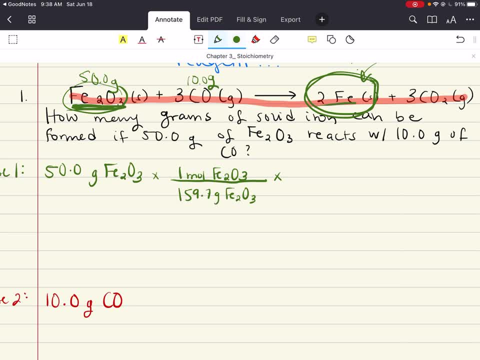 One mole of iron oxide gives you two moles of iron here. This is what I meant, right, Because we're looking at the product. So that is, we're going to use this relationship here, All right, And so this is the mole to mole ratio we're going to use. Remember, you can get this mole to mole ratio. 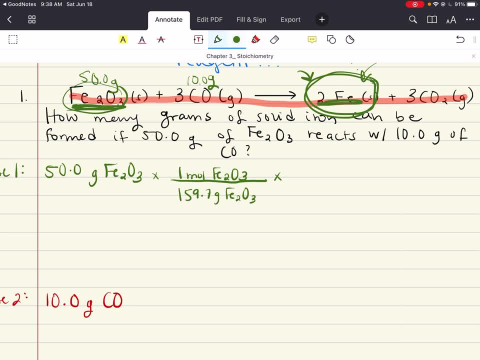 either from the chemical formula or from the balanced equation. Now we're trying to find a limiting reagent. So you're looking at the whole equation: One mole of iron oxide gives you two moles of iron. This equation was balanced for us, So we're going to use those numbers. 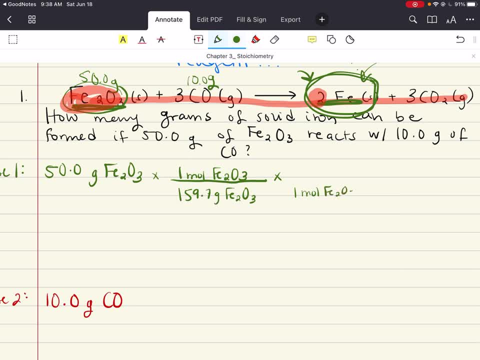 and we're going to write: one mole of iron oxide gives us one mole of iron. Now we want to know at the end of the equation we're going to write: one mole of iron oxide gives us one mole of iron, How many grams are we getting as a final product of just solid iron? So we need to do one more. 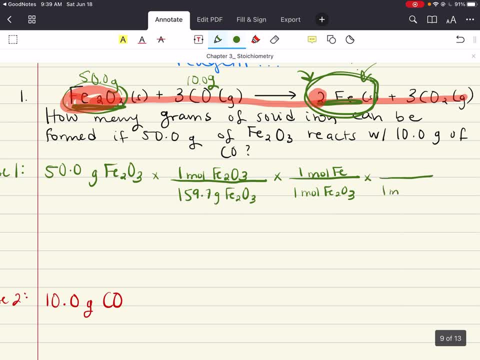 conversion, again using the, the idea that a mole relates to mass. One mole of iron should be equal to the molar mass of iron, which is 55.85 grams of iron. All right Now notice. notice how everything cancels out Grams of iron oxide. cancel out Moles of iron oxide. cancel out Moles of iron. 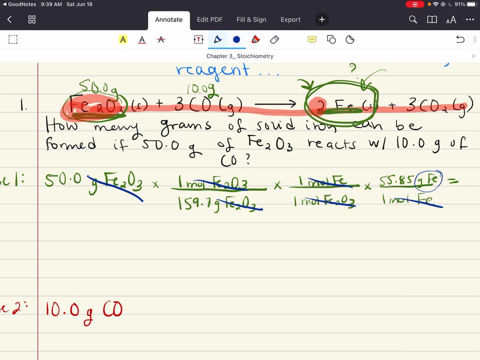 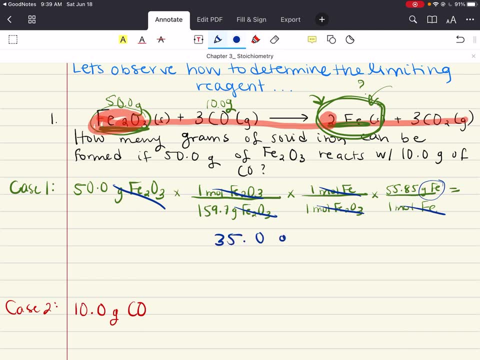 oxide cancel out, And our final leftover unit is grams of iron. And if you were to calculate all this using a calculator, you would get 35 grams of iron. So from the 50 grams of iron oxide you would be able to produce 35 grams of iron. All right, Now we want to calculate also how much. 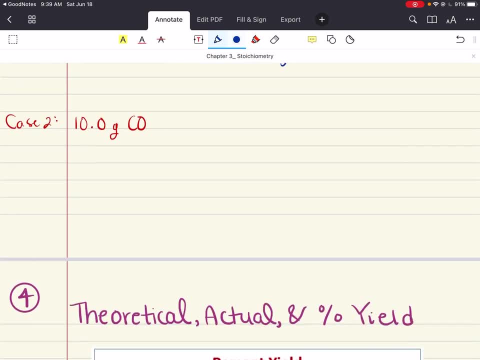 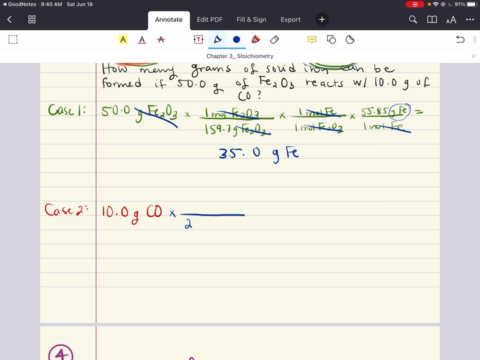 do we get if we use carbon monoxide? Same idea here. We're going to start off with 10 grams of carbon monoxide. Carbon monoxide has a molecular weight of 28.1 grams. That's going to be equal to one mole of carbon monoxide. right, Because, remember, our mole relates to mass. All right. 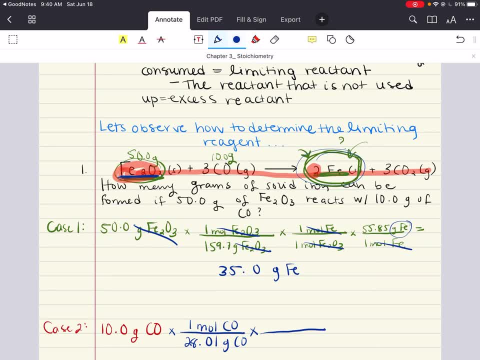 Then we're going to do a mole to mole ratio. We have three moles of carbon monoxide in our balanced equation and we have two moles of iron, And that is our goal: to find out how much iron we are forming. So we're going to write three moles. 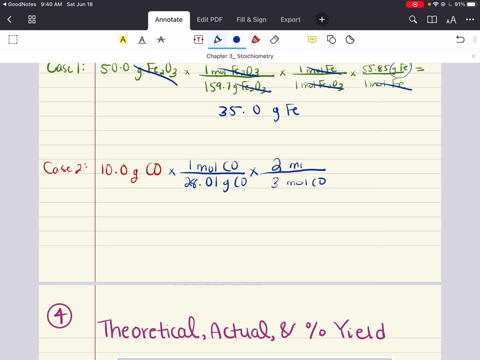 Carbon monoxide two, Two moles of iron, And then we're going to do our final conversion because we want to know how much grams of iron. So one mole of iron is equal again to 55.85 grams of iron. All right, Notice. again, everything cancels out Grams of carbon monoxide, moles of. 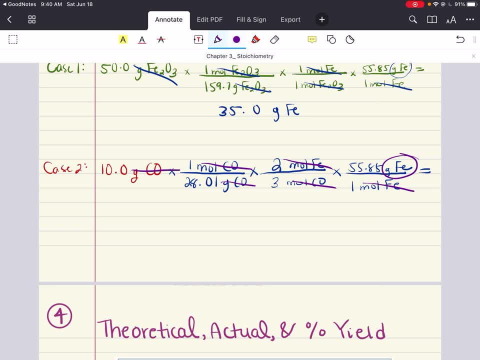 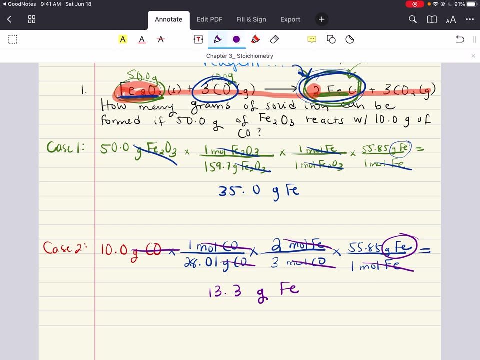 carbon monoxide moles of iron, And our last final unit is going to be grams of iron. Perfect, If we calculate this, what we get is 35 grams of iron, And then we're going to do our final conversion: 13.3 grams of iron. So the 10 grams of carbon monoxide is able to produce 13.3 grams of iron. 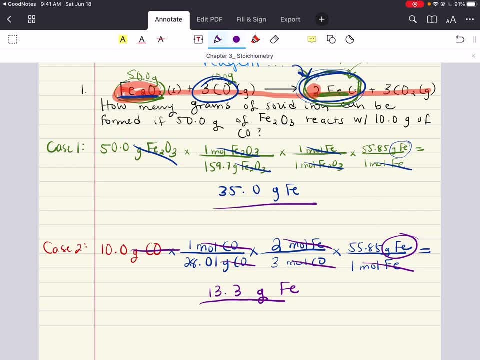 total. Now, which one is less? 35 or 33?? Obviously 33.. What that means is our limiting reagent is going to be carbon monoxide. We can only produce as much iron as there are of the limiting reagent, And the limiting reagent is carbon monoxide. 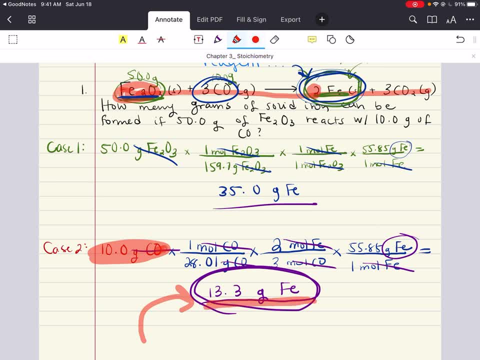 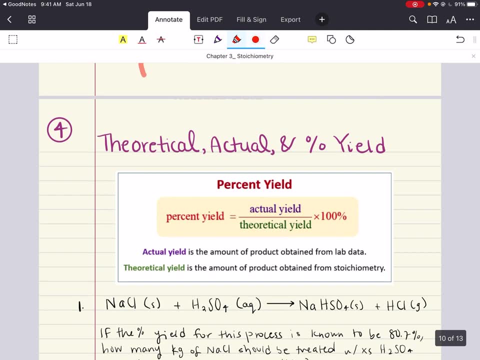 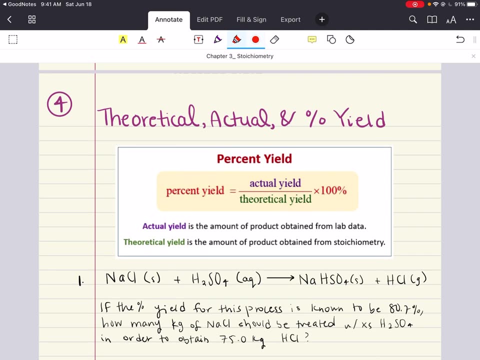 Because it produces a lesser amount of iron than the iron oxide- Fantastic. Now, one important topic that we're going to cover here in this chapter that is also going to be super crucial for your general chemistry lab course- is understanding the difference between theoretical, actual and percent yield. 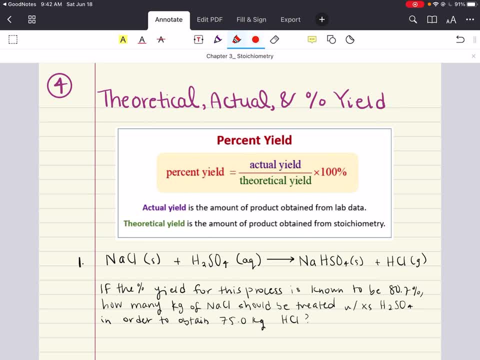 Whenever we use stoichiometry to predict the amount of product that should be obtained, this quantity is going to be our theoretical yield. Theoretically, if everything went well in the reaction- no errors in preparation or transfer or anything of the sort. this is how. 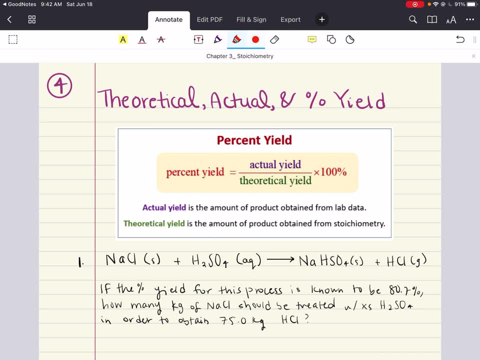 much product we should get. Now, the actual amount obtained at the end of your experiment that you measure, that's your actual yield And that's how much product we should get. So we're going to measure the actual amount obtained at the end of your experiment And that's going to be our theoretical yield. 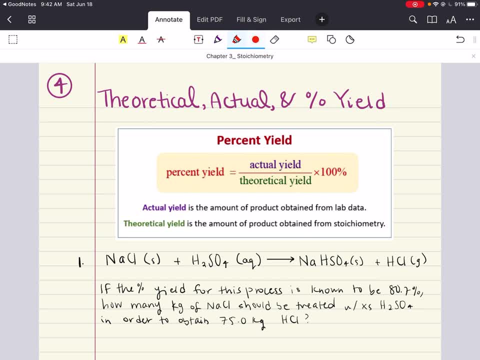 And it's going to usually always be less than the theoretical yield because of human error, instrument error and so many other factors that can occur that might lower your yield during an experiment. Now the percent yield of a reaction is a useful way to relate. 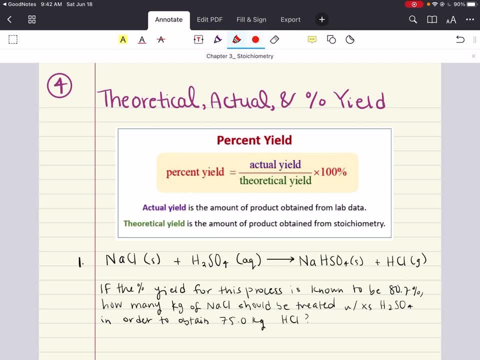 actual yield to theoretical yield And it has the following expression: Percent yield is actual yield divided by the percentage of product that is obtained And that's the actual amount obtained, And that's by your theoretical yield times 100 percent. all right, so this is something that you might be. 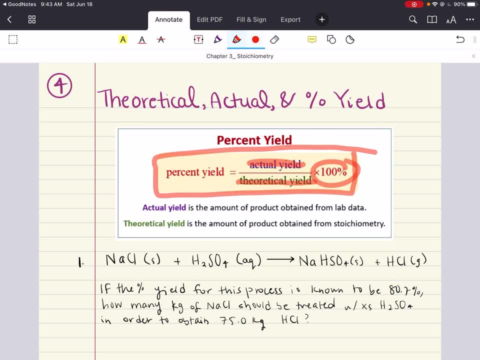 asked to always calculate at the end of experiments you might do in general chemistry, so it is important that you know how to do it. all right, and we're going to practice by doing a example problem, all right, so this is our example problem. we have um this equation that 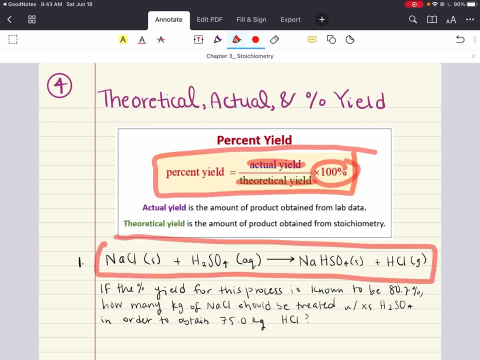 we are given. all right, hydrogen chloride gas is going to be made by reacting- reacting sodium chloride with concentrated sulfuric acid. all right, cool beans. now, if the percent yield for this process is 80.7 percent, how many kilograms of sodium chloride is going to be made by reacting sodium chloride with concentrated sulfuric acid? 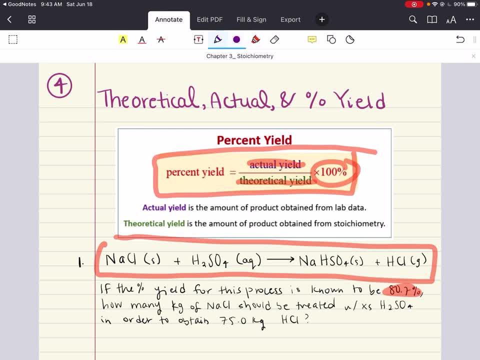 Chloride should be treated with sulfuric acid to get 75 kilograms of hydrogen chloride. All right, so that's our problem. If the percent yield for this process is known to be 80.7%, how many kilograms of sodium chloride should be treated with excess hydrochloric acid in order to obtain 75 kilograms of hydrogen? 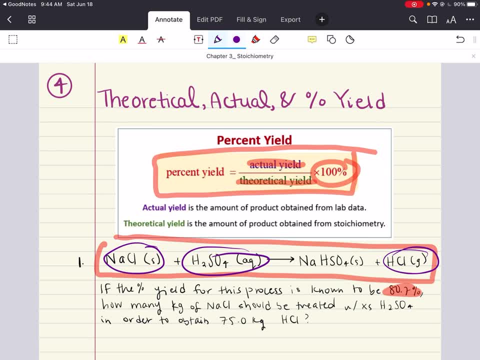 chloride. Now, 75 kilograms of hydrogen chloride represents the actual yield. all right, how much you would actually get at the end of your experiment? all right, So that's an important thing to make sense of this problem. So you can think about it as if the percent yield for this process is known to be 80.7%. 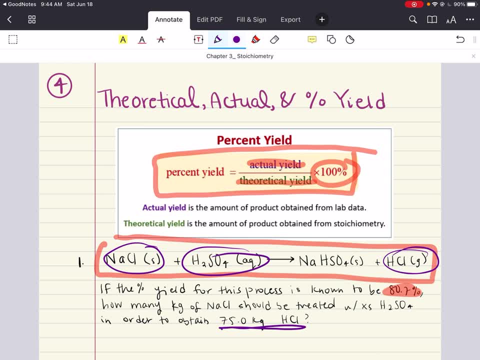 if the percent yield for this process is known to be 80.7%, how many kilograms of sodium chloride should be treated with excess sulfuric acid in order to actually actually experimentally obtain 75 kilograms? So this understanding of this problem and what this value entails is important, right. 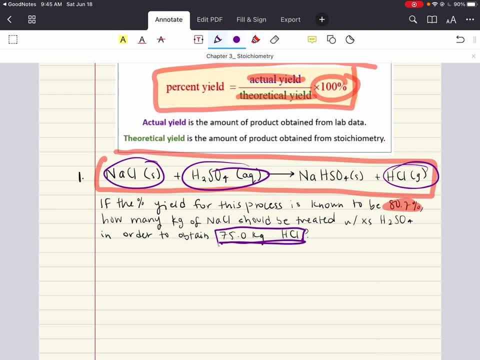 Because you're going to be calculating percent yield and so you need to understand what your actual yield is. So the first key for sodium percent yield problems is to use the equation defining percent yield. all right, And so we know what the we know what the actual yield is. all right, 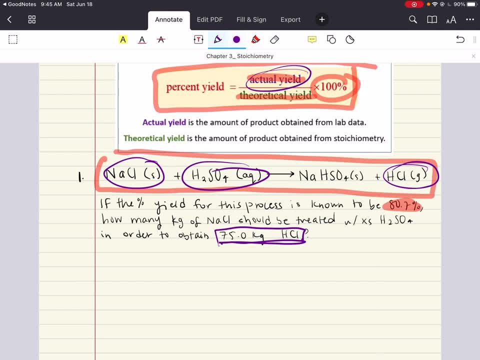 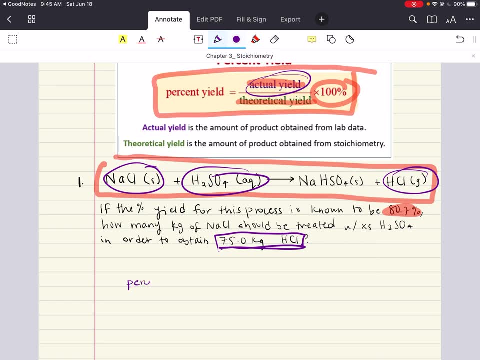 And we know what the percent yield is, So we can actually use this to get the theoretical yield. So let me show you what that means. Let me rewrite percent yield, all right. equals actual yield over theoretical. So let me rewrite percent yield, all right. 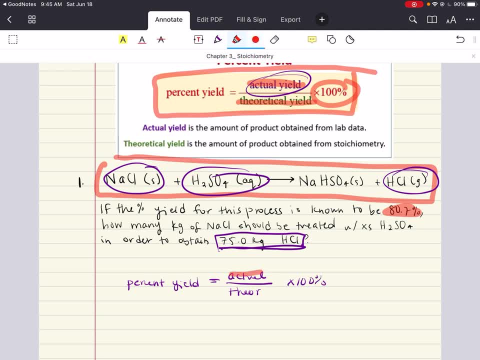 Times 100%. Now we know our actual yield. It's 75 kilograms of hydrochloric acid- Beautiful. We know what our percent yield is too. They give this to us: 80.7%- Cool. We can use this equation, still through rearranging, to find our theoretical yield. 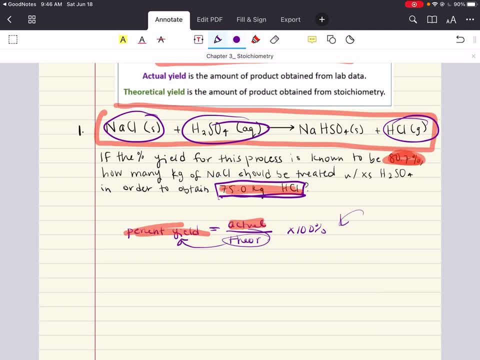 All we have to do is move things around, move the theoretical yield here and move the percent yield down here, So then our theoretical Yield is going to be equal to our actual yield over our percent yield times 100%. And if you plug this into a calculator, what you're going to get is 92.9 kilograms of hydrochloric. 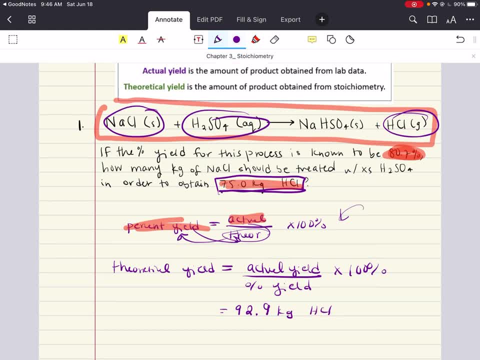 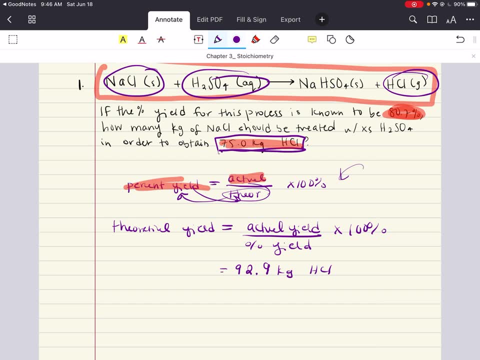 acid. All right. The second key is knowing that the theoretical yield always involves a stoichiometry, Stoichiometry calculations. So, since we know the theoretical yield, we can use a stoichiometry problem to determine how much sodium chloride is required to result in that theoretical yield of hydrochloric. 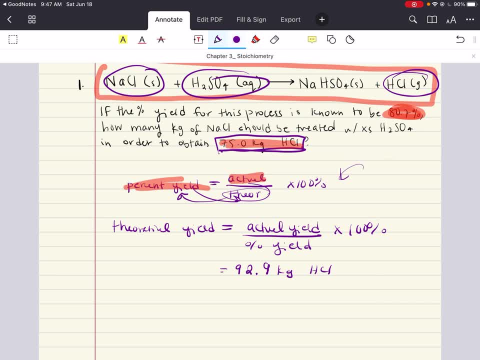 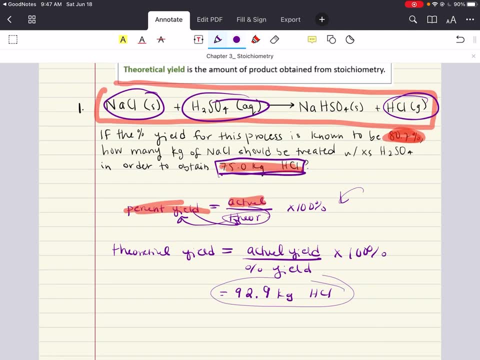 acid, All right. So that's exactly what we're going to do now, because the problem doesn't ask us just our theoretical yield. It wants to know how much sodium chloride should be used. All right, How many kilograms of sodium chloride? 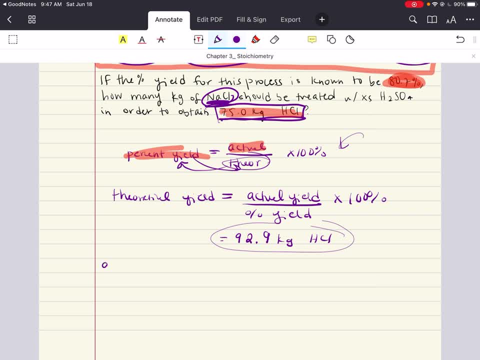 So that's what we're going to figure out. We're going to start it off by writing 92.9 kilograms, but we're going to write it in grams, So 10 to the 3 grams of hydrochloric acid. All right, 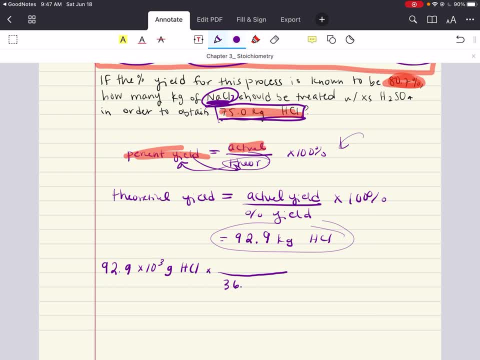 And we're going to use a conversion. What's? the molar mass of hydrochloric acid is 36.46 grams of hydrochloric acid is equal to 1 mole of hydrochloric acid. Remember, mole refers to mole Um. 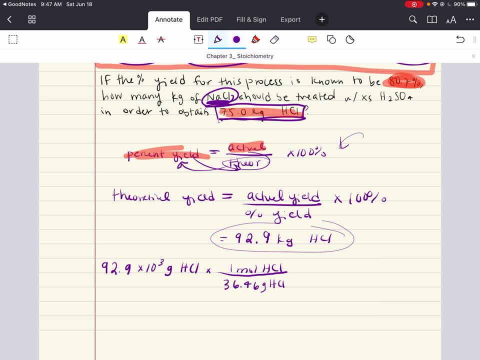 Mole relates to mass, So you can use this conversion. Next, we're going to use a mole to mole ratio, right, Because we don't want any more information about hydrochloric acid. We want to know how many kilograms of sodium chloride. 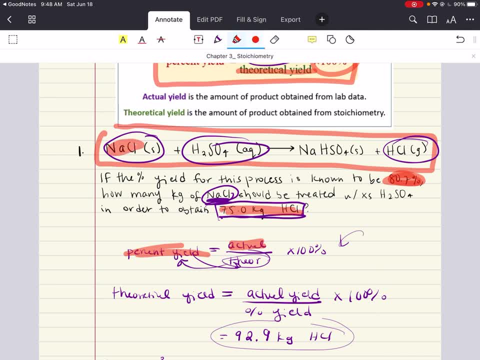 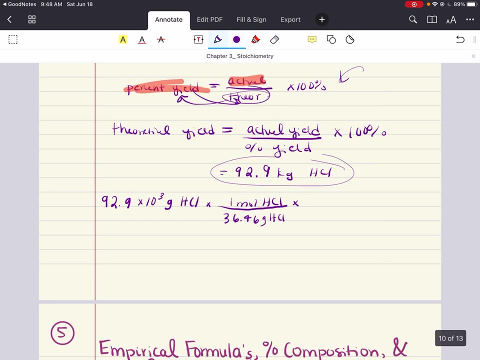 We're going to look back at our equation. What's the coefficients associated with these two molecules in our balanced equation? 1 mole of sodium chloride to 1 mole of hydrochloric acid. Those are the coefficients associated here, Just ones. So that is what we're going to use: 1 mole of hydrochloric acid to 1 mole of sodium chloride. 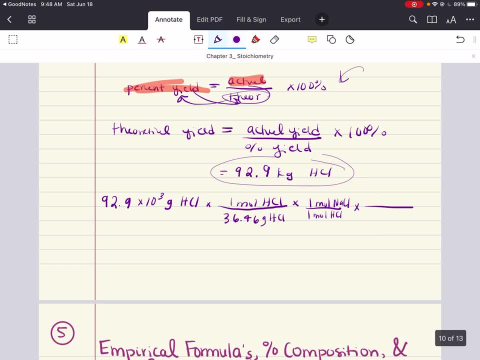 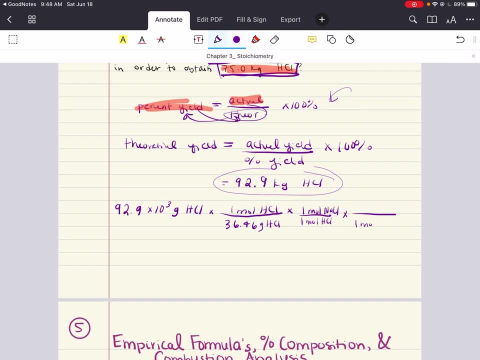 All right, And for our final conversion, we want grams of. we want grams or kilograms of sodium chloride. So we're going to write that 1 mole of sodium chloride results in 58.44 grams, because this is just the molar mass of sodium chloride. 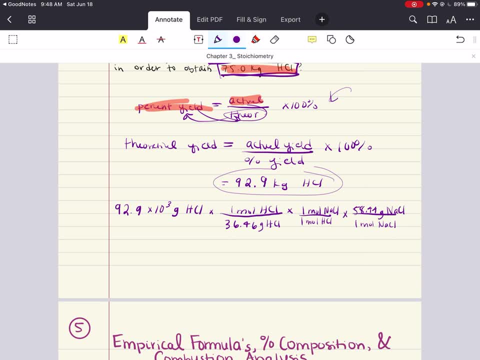 And then if we plug this in, And then if we want to get kilograms as a final number, we can do one more conversion: Just converting grams to kilograms, 10 to the 3 grams, is equal to 1 kilogram. And then if we plug all of this into our calculator, what we're going to get is 149 kilograms of sodium chloride. 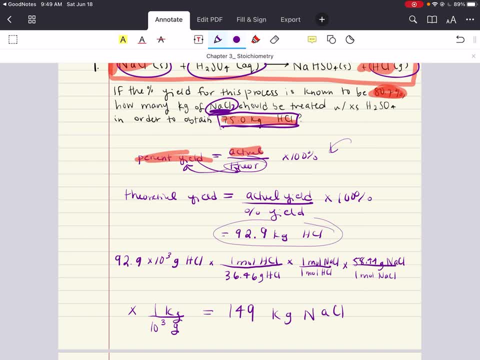 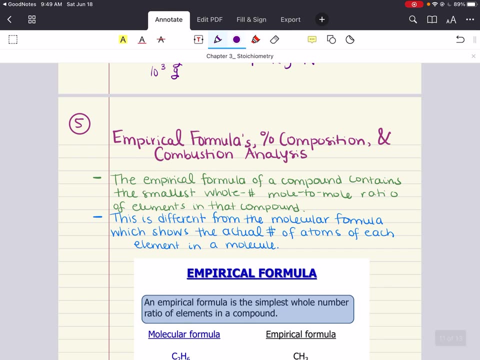 All right. so we would need this much sodium chloride in order to Obtain 75 kilograms of hydrochloric acid as a product, as an actual yield- Fantastic. Now on to our final topic. Finally, we want to talk about empirical formulas, percent composition and combustion analysis. 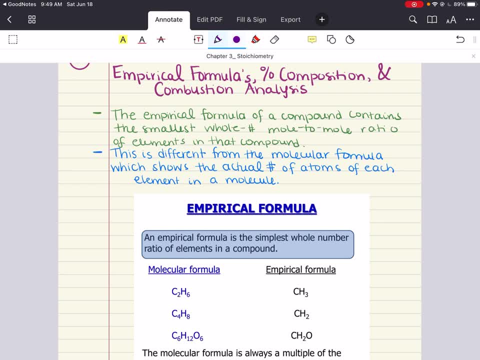 Now, the empirical formula of a compound contains the smallest whole number- mole to mole ratio- of elements in that compound. This is often different from the molecular formula which shows the actual number of atoms of each element in a molecule. So if the empirical formula and the molar mass of a particular compound are known, 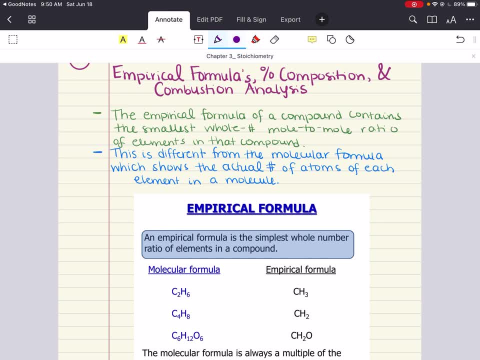 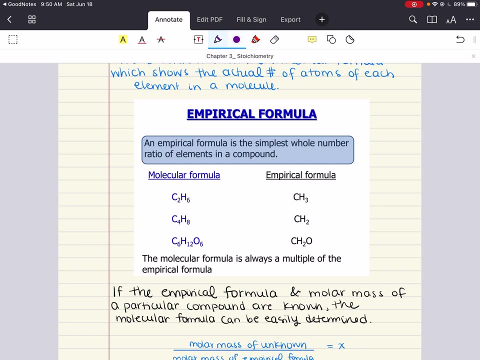 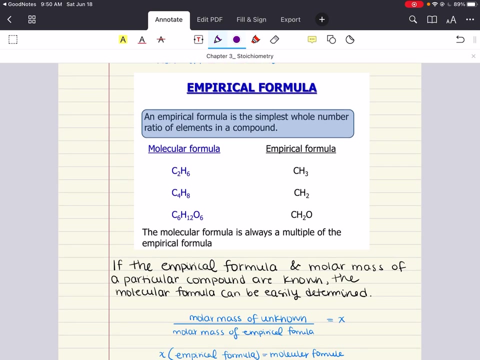 The molecular formula can then easily be determined. Now, a molecular formula will always be a whole number, multiple of the number of atoms in the empirical formula. So Another way to describe The composition of a compound is going to be in terms of percent: composition by mass or mass percent. 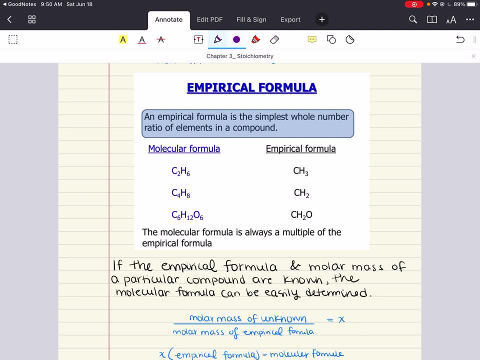 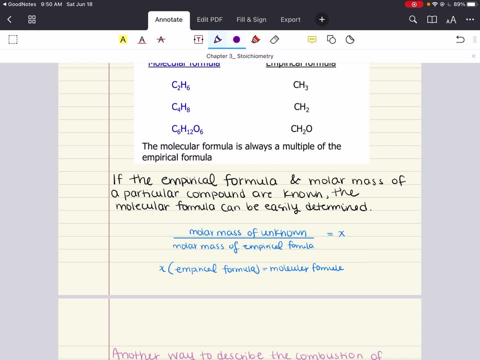 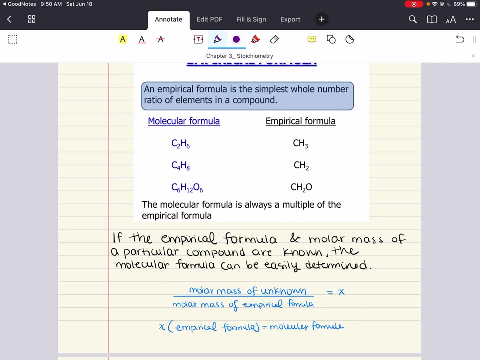 We're going to cover the formula for this Right here. molar mass of unknown Over a molar mass of empirical formula equals X. So if the empirical formula and the molar mass of a particular compound are known, The molecular formula can be easily determined. 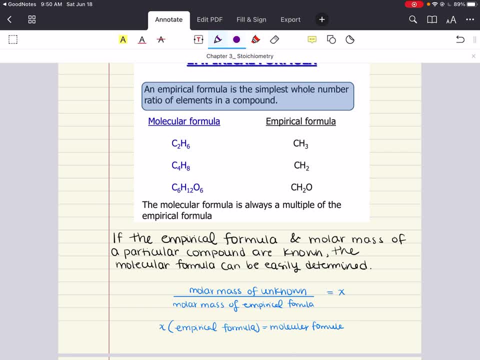 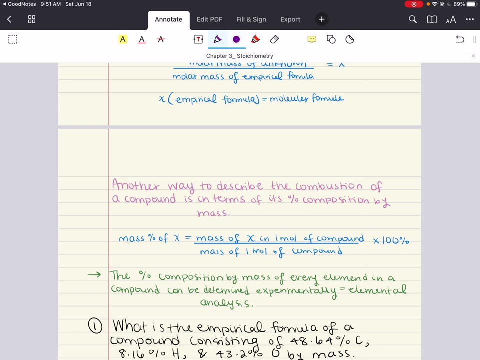 All right. and the another way to describe the composition of a compound is in terms of its percent: composition by mass, or mass percent. Now, the percent composition by mass of every element, of every element in a compound, can be determined experimentally through a process referred to as elemental analysis. 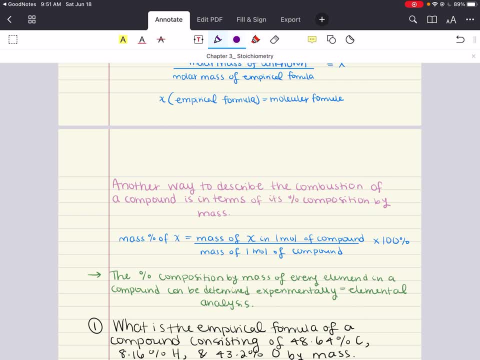 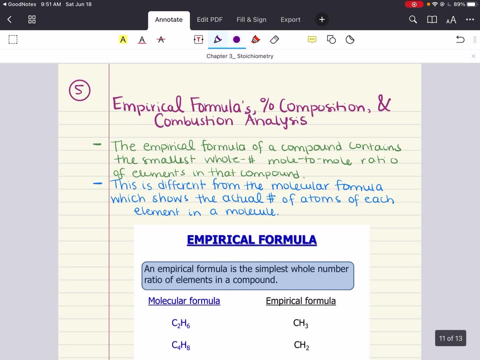 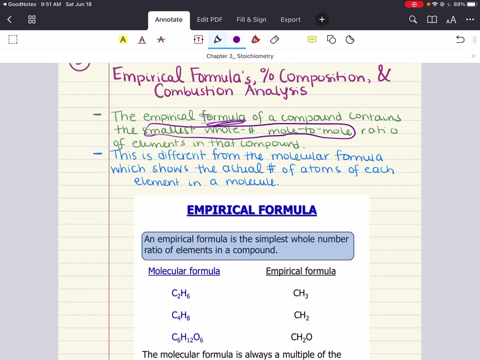 Once percent composition know is known, It can be used to determine The extent of the amount of atoms present in a molecule. So let's go ahead and start studying this empirical formula. So one more time- I just think this is important to repeat. the empirical formula of a compound is going to contain the smallest whole number, multiple ratio, of the elements in that compound. 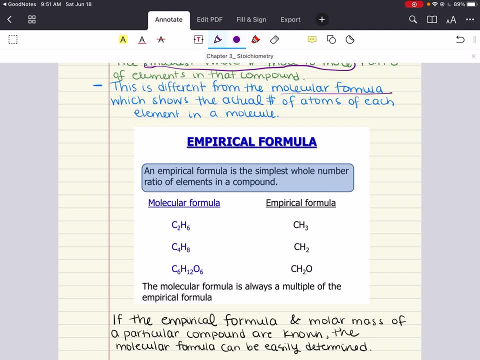 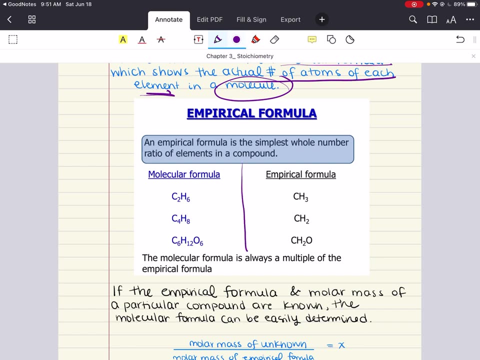 This is different from your molecular formula, where you know the actual number of each Adam present in an element in a molecule. You can know the actual number of atoms of each element in a molecule, All right, so here's a cool way to look at this, right. An empirical formula is the smallest whole number ratio of elements in. 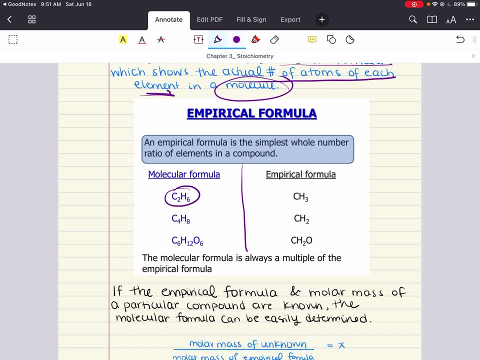 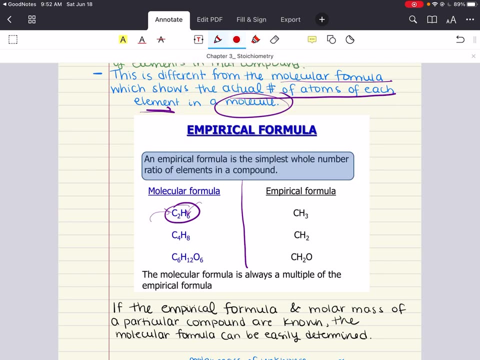 a compound. This is your molecular formula. You're going to have in this molecule two carbons, six hydrogens. That's the molecular formula. The empirical formula, however, is the smallest whole number, mole to mole ratio. So what you can do is each one of these numbers right here. 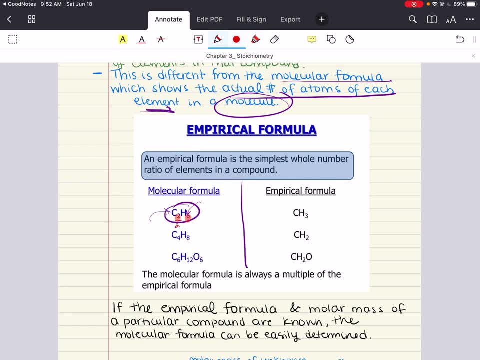 can actually be divided by two, And when you divide each one by two, you get C1H3.. This compressed form, this is referred to as the empirical formula, All right, And the molecular formula is always a multiple of the empirical formula, All right, So that's really important. 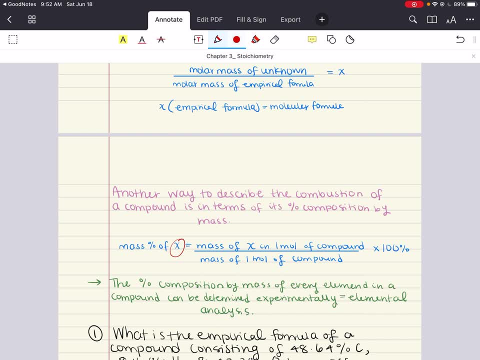 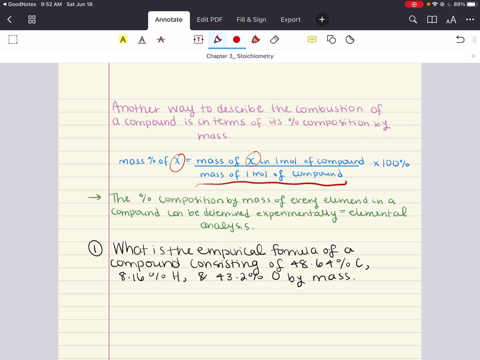 to note Now the mass percent of X of an element in your molecule. it's going to be the mass of X in one mole of compound over mass of one mole of compound, And this present composition by mass of every element in a compound can be determined. 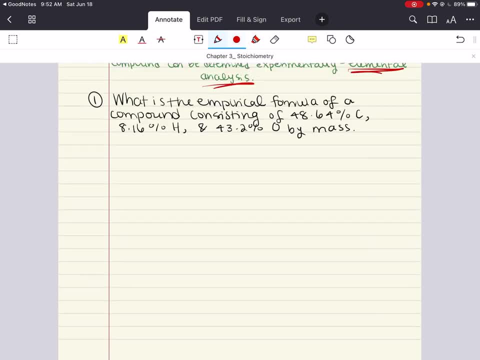 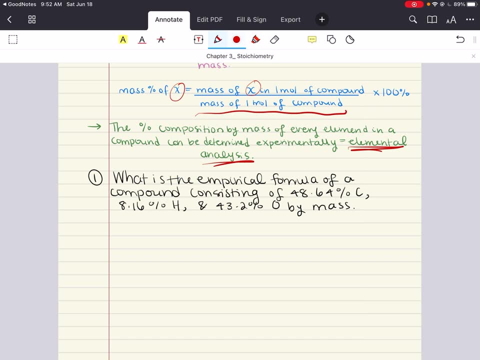 experimentally, So that's also important to know. So, with that being said, I think the best way to really get the hang of this is let's actually do a practice problem together, All right? This practice problem says what is the empirical formula of a compound consisting? 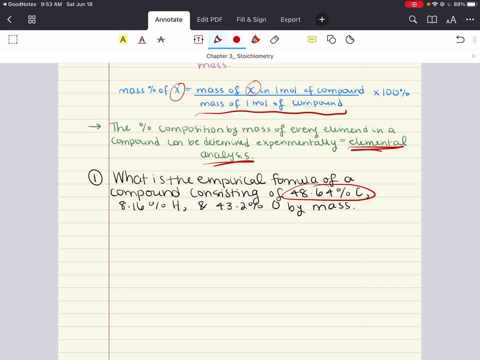 of X and Y And what is the empirical formula of a compound consisting of X and Y? And what is the of 48.64% carbon, 8.16% hydrogen and 43.2% oxygen? All right, Keep the following two ideas. 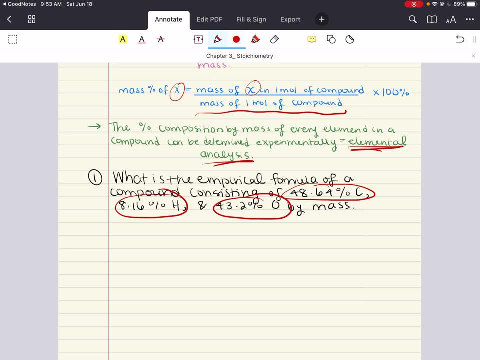 in mind as we solve this problem. One percent composition is percent by mass, And two, remember our empirical formula- is the smallest whole number: mole to mole ratio. All right, So when the percent composition is percent by mass and two, remember our empirical formula- is the: 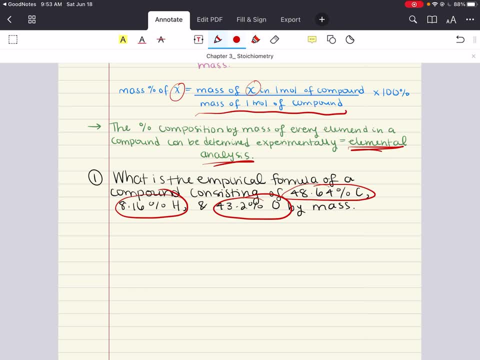 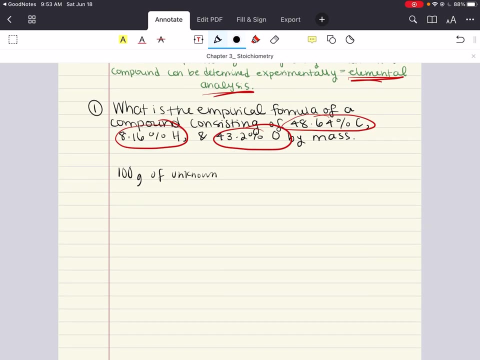 percent composition by mass is given, it's going to be the easiest to assume that we have 100 grams of this unknown compound total. So we're going to assume we have 100 grams of this unknown compound, All right. Which means we can say the following: 48.64% carbon is really. 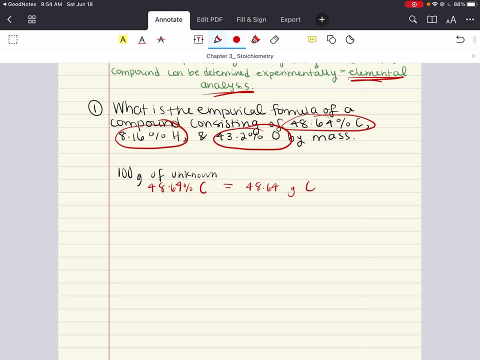 just 48.64 grams of carbon, because we have a total of 48.64% of carbon. So we're going to assume that we have a total of 100 grams of unknown 8.16%. hydrogen is really we can talk about it now as 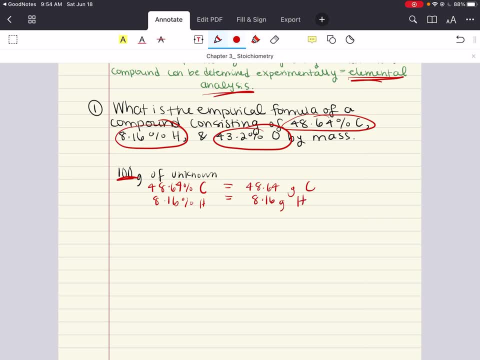 8.16 grams of hydrogen, because we're assuming 100 grams of unknown, And same for this oxygen, 43.2% of oxygen. we can just now think of it as 43.2 grams of oxygen. Now we can take advantage of. 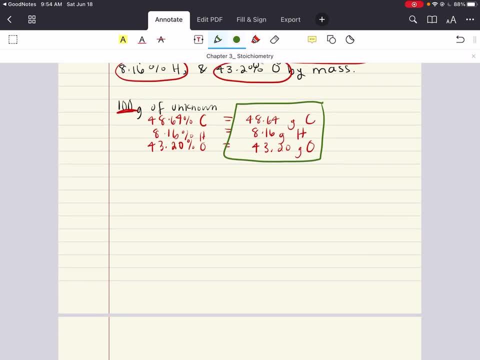 this to calculate the moles of each. How are we going to calculate the moles of each? How are we going to do this? Well, we can find out the moles of the number of moles of carbon simply by doing taking 48.64 grams of carbon and doing a quick mole to mass ratio, So 12.01 grams. 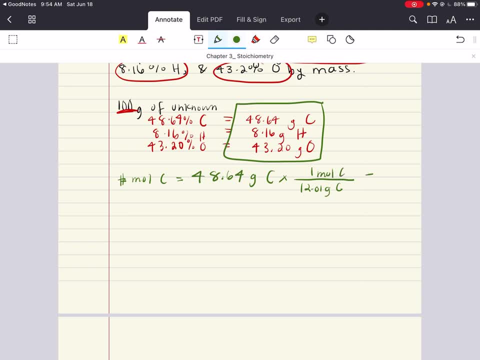 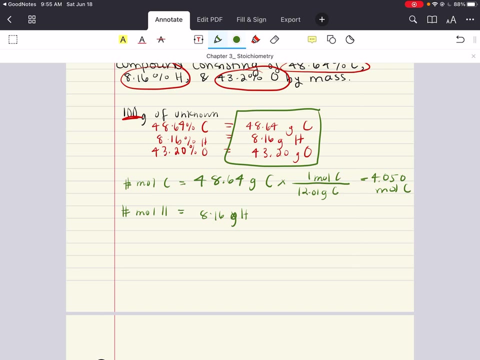 of carbon is equal to one mole of carbon. That gives us 4.05 mole carbon. And we could do the same for number of mole of hydrogen. Same thing: 8.16. grams of hydrogen times. what is the molar mass of hydrogen? 1.008 grams Hydrogen is one mole of. 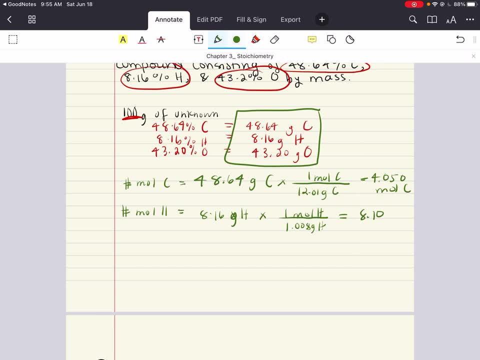 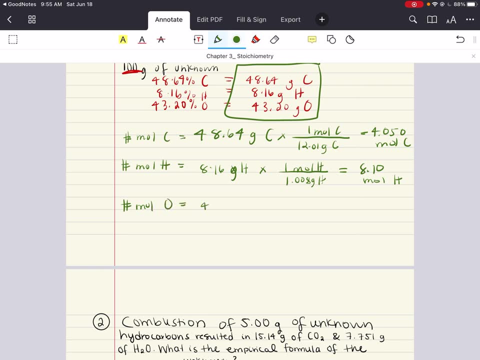 hydrogen. This gives us 8.10 moles hydrogen. And, last but not least, we can do this for oxygen as well. We have 43.2 grams oxygen. 15.999 grams oxygen to one mole: We get 2.2 grams of oxygen. 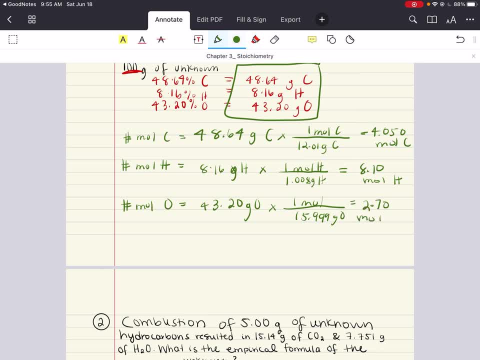 We get 2.70 moles oxygen. All right, Awesome. So then an empirical formula- remember, let's go back to this definition- is the smallest whole number, mole to mole ratio. So, now that we have these moles of each atom, we need to divide the number of moles of each atom by the smallest number of moles. 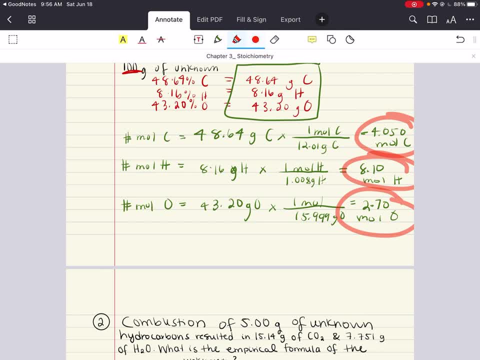 so we can get this mole ratio. So we have 4.0 grams of oxygen, We get 2.0 grams of oxygen, 4.05 moles of carbon, 8.0, 8.10 moles of hydrogen and 2.7 moles of oxygen. Which one of these is? 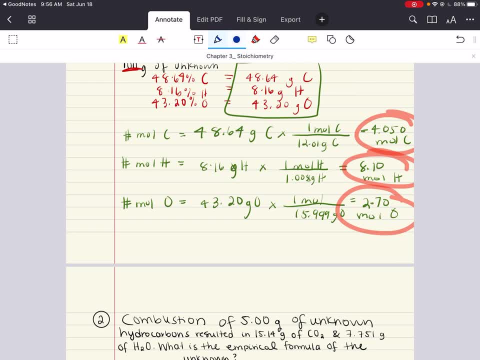 the smallest number, 2.70.. So we're going to divide each one of these numbers by 2.70.. All right, Each one of these numbers by 2.70.. For carbon, when you divide, you're going to get 1.5.. 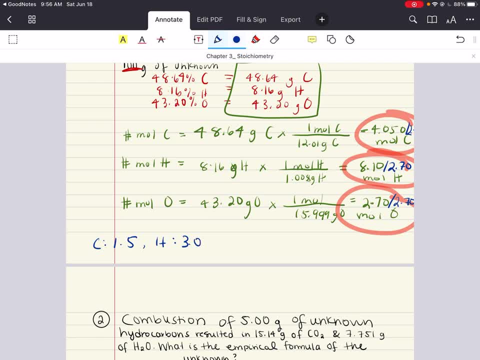 For hydrogen it's going to be about 3. And for oxygen it's obviously just going to be 1.. All right, Fantastic. So that means the whole number ratio is going to be 1.5 to 3 to 1.. So that: